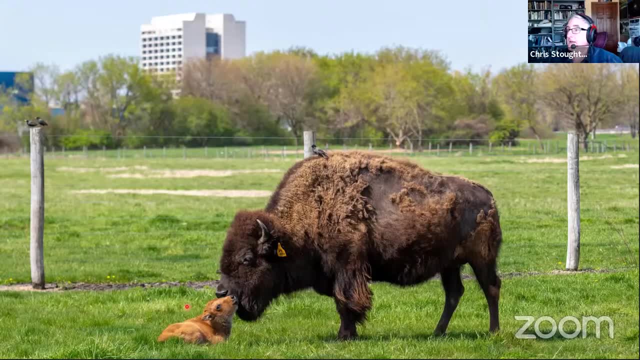 And just for perspective. I'll be showing more pictures of the lab later. This is the famous high-rise building. I'll show you a picture. This is sort of looking out the front of it and we'll look out the backyard. So that's the general orientation and welcome to Fermilab. 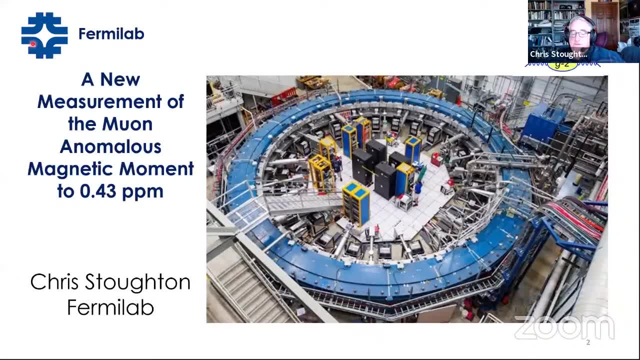 This is the experiment. The G-2 experiment looks like this and instead of so many experiments where you see a little drawing of a person, we have an actual person standing in the middle to give you an idea of what the scale is. This is a typical raised platform computer floor here electronics rack. 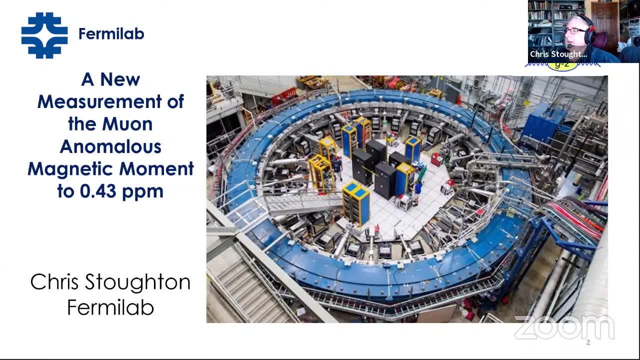 And this big blue thing is the storage room that we store the muons in while we make the measurement, and the upper left-hand corner is the lead-in of where the muons come in from. So that gives you a basic orientation of where you're standing. 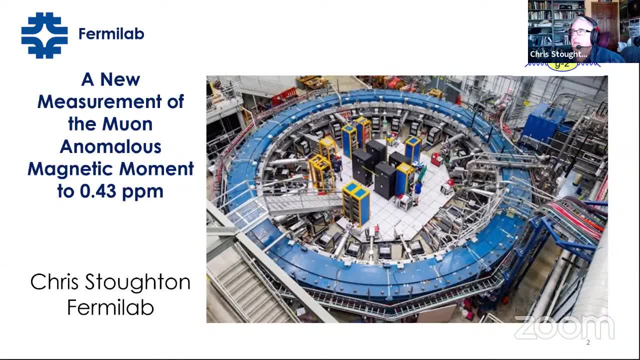 The entire experiment is measuring. this Feynman diagram-like thing we have drawn as our logo. It graphically demonstrates illustrates what we're measuring. that is, muons interact with a static magnetic field and have a certain reaction stream. If it was just this point, g would be exactly two. 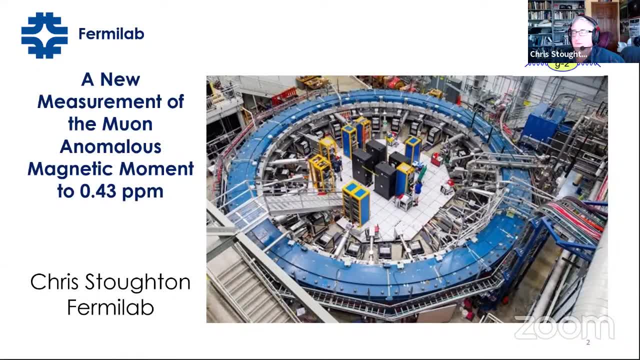 and g minus two would be zero and there wouldn't be much of an experiment. As we know, virtual particles take shortcuts in this interaction and it's correctly. summing up all of the different contributions to the interaction is the theoretical challenge, and the experimental challenge is measuring that effect. So I really like experiments where the 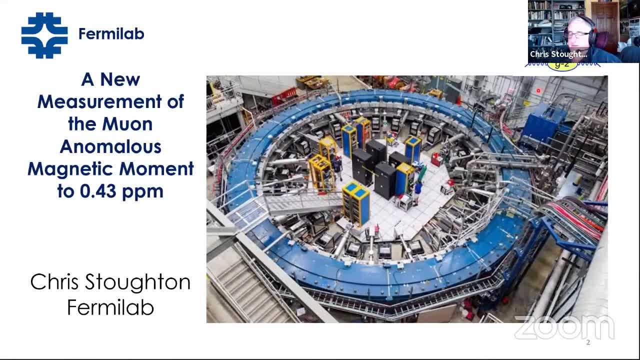 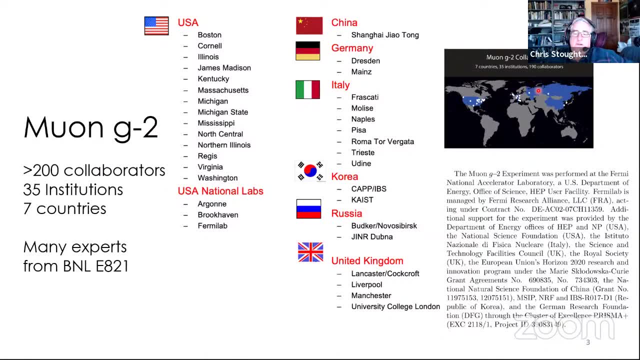 logo is a summary of the experiment, so you don't have to go back and forth. Okay, I want to emphasize, of course, that this is not my talk, but it's the result of, well, hundreds of people working for decades around the globe to get this result. And, just by the way, 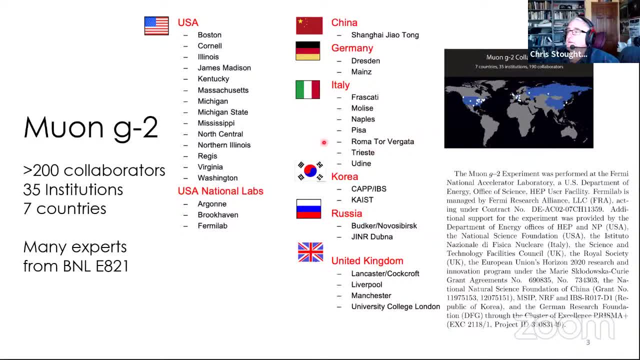 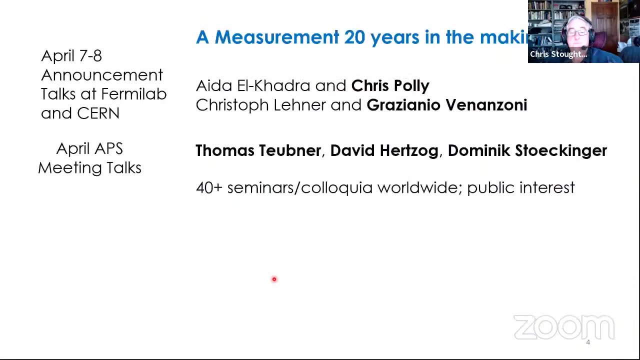 one tip in case there are any young researchers out there who haven't yet chosen a collaboration or a career. not that this is why I joined the experiment, but if you are on an experiment with Italians, they have the best collaboration, In my humble opinion. Okay, So it's a measurement 20 years in the making, And in April 7th and 8th. 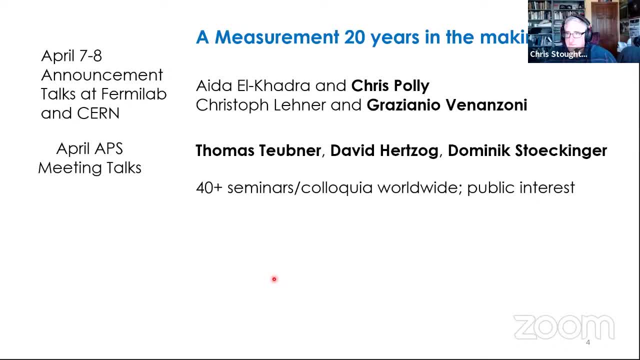 of this year. there was the announcement at Fermilab and at CERN, more or less coordinated, explaining what we saw. Chris Polley gave the results at Fermilab and Graziano gave the results at CERN, Speaking with theorists. Aida and Christoph are two theorists that have been working very 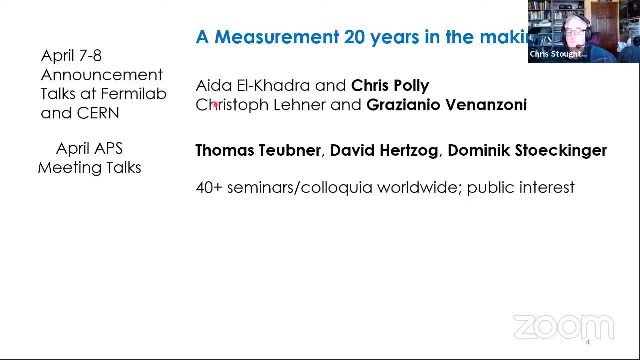 closely to come up with the prediction of what we should see. And then, at the American Physical Society talks a few weeks later, Thomas, Dave and Dominic also gave talks. So if you want to look up more details, you can find their talks, And this number is probably a little bit low. 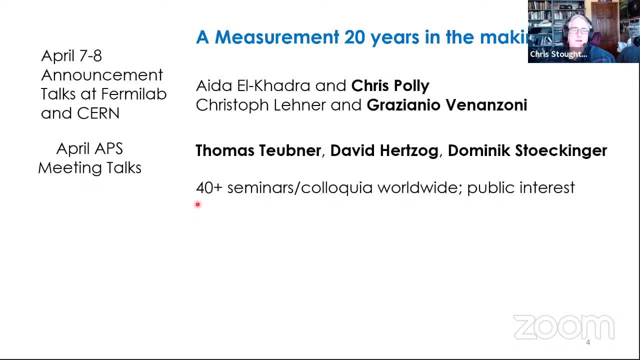 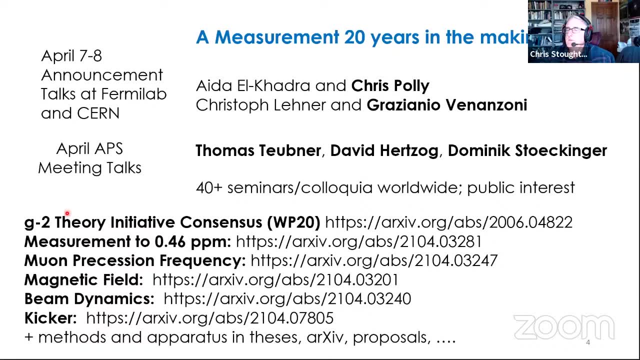 I bet we're up over 100 seminars now And indeed some not small amount of public interest. If you want to really see what we did, not just rely on the story, I'm going to tell you there are five core papers that you should read, And I put this one in the so-called kicker paper. 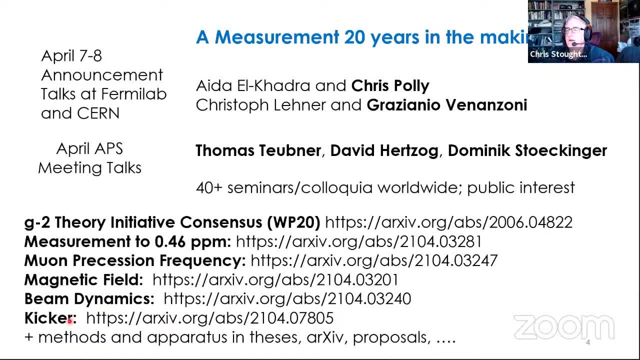 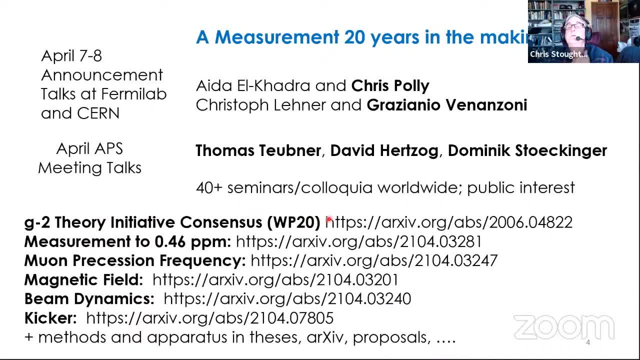 And this is the first paper that I wrote, And this is the first paper that I wrote- value of the calculated value for a sub? u that we can calculate. This paper overviews the measurement technique. It's mostly what I'll talk about today, And then there are three basic parts. 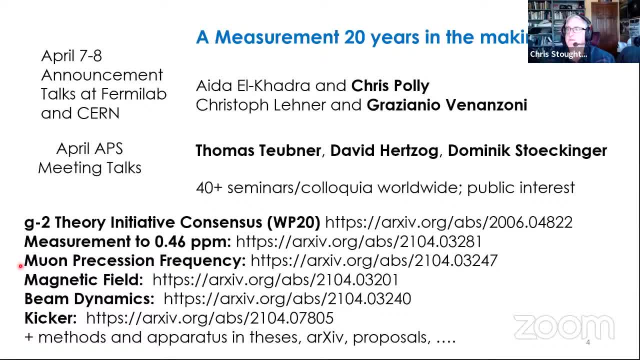 of the experiment that combine measuring the actual precession frequency, measuring how strong the magnetic field is, and then finding out where the beam is. since the magnetic field isn't the same everywhere, You've got to find out exactly where the beam is. And then this kicker paper is. 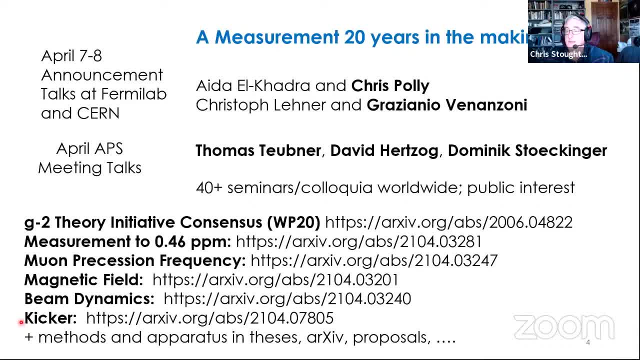 also out which describes an important part of the apparatus We have. I think the tracker paper is under review now by the collaboration And there's plenty of methods and apparatus, talks and theses on the archive And indeed the proposal stands up as a pretty good document as to what our basic 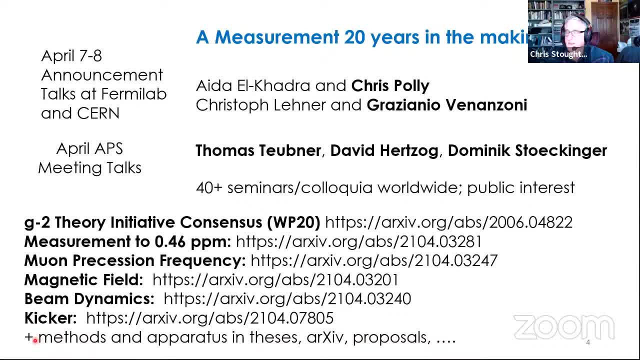 methods are. I think it's not this year, But last year's thesis award at Fermilab was the thesis measuring of the muon precession frequency. Okay, so I'll cut to the chase here. let you know what the big deal is. 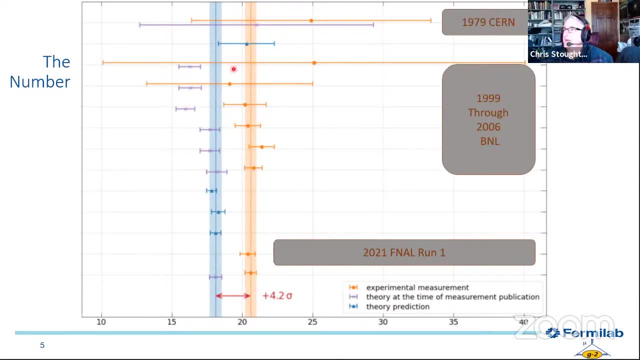 As a function of time. this number has been measured many times, So time goes more or less down. Actually, back in 1959, 1960, Leon Lederman made some early measurements, But those were like 1%, So the error bars would be huge on this scale. The scale left and right is just a couple digits out in. 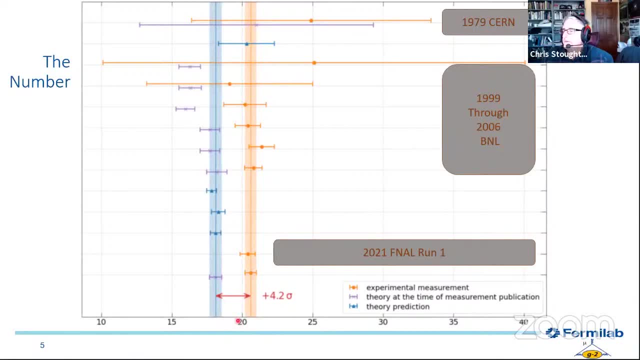 significant figures, significant digits, So they're all scaled to be on. so they all fall on this plot nicely. And you can see back in the 1979 CERN experiments there was sort of gross agreement between theory- I'm sorry, theory here on the left- and what, what the experiment measured. 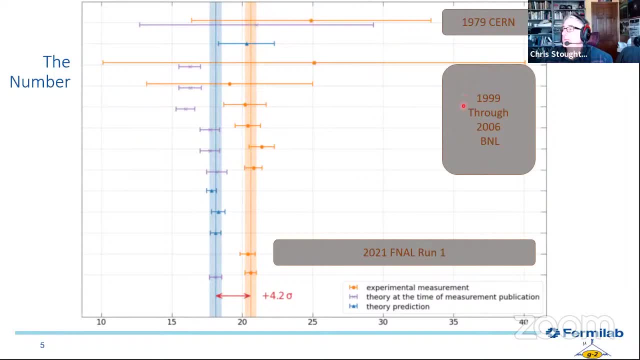 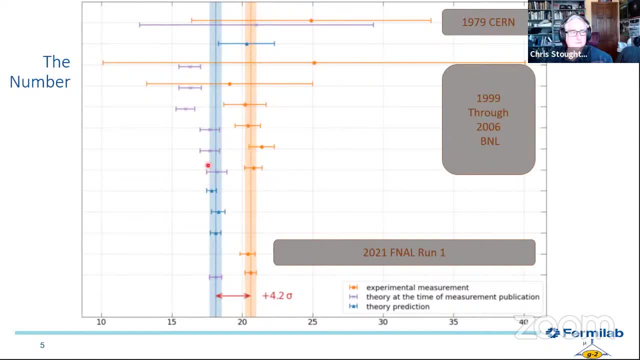 And it's this difference here, finally published in, I think, 2006,. that had a few sigma difference. That was the anomaly that people talked about and wondered about, widely cited, And this was the motivation for us to go ahead and move the main storage ring. 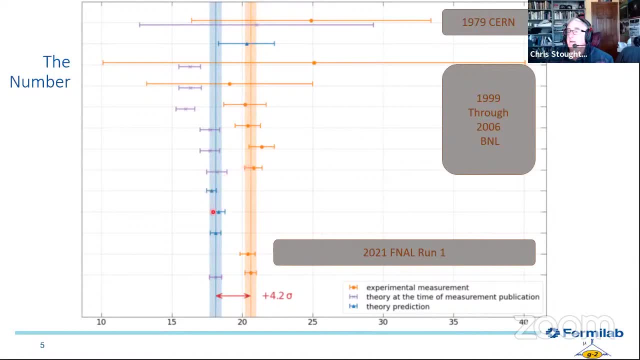 apparatus to Fermilab. Meanwhile, theorists kept calculating, getting better and better error bars right, And this is the new number we made. So all the work over the past decade, in the last decade, will tell you about, I think, the kind of 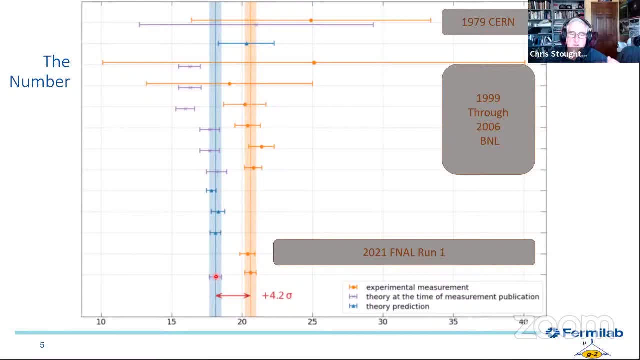 the number that we made right. I didn't get to the one that I had during the analysis, but it's a football field in your country. is football, football or football? 100 yards, right To 0.46 parts per million, it's like the width of a human hair. So if you're a referee making an off-sides, 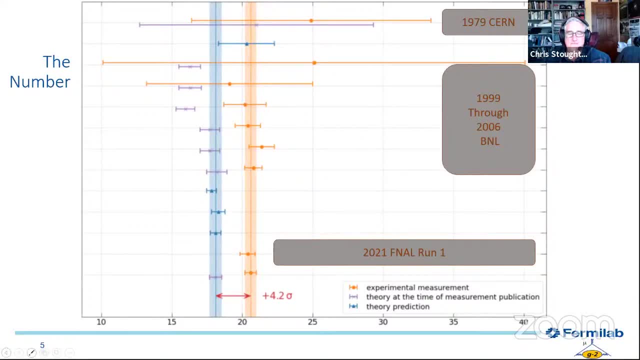 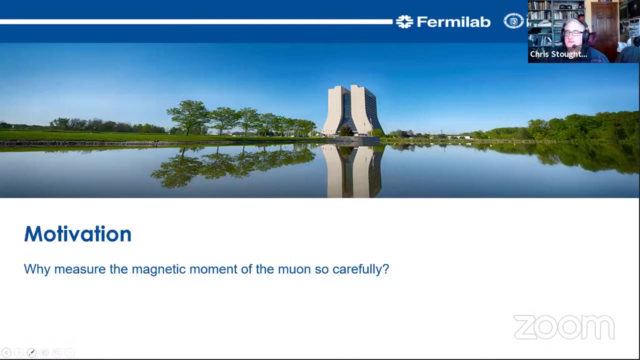 call. hopefully they won't ask you to be that sensitive. It's just nice to step back for a second when you ask: why did it take so long? Because measuring things carefully takes a long time. Okay, so let's step back for a second and consider: why would you bother measuring the 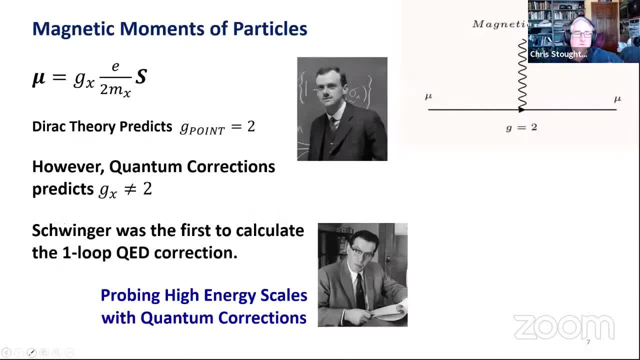 magnetic moment of the muon. What possible use is it right? So, magnetic moments of particles. if you think back to your quantum field theory class, or really quantum mechanics class, the Dirac theory, the Dirac equation predicts that the magnetic moment 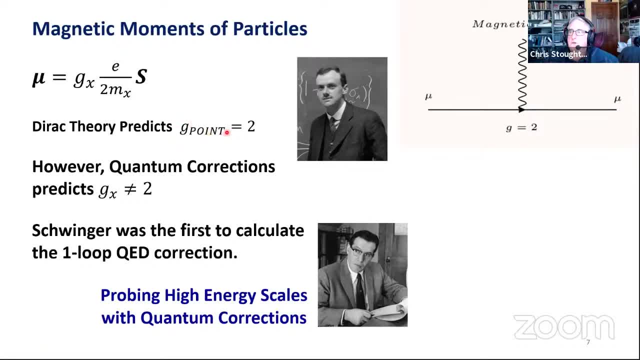 of a simple particle, which is also called a point particle, is exactly two right, That is the ratio between its magnetic moment, how fast it processes, and its spin, which is one half in the case of the muon. right Actually goes with this geometric factor of two, the so-called 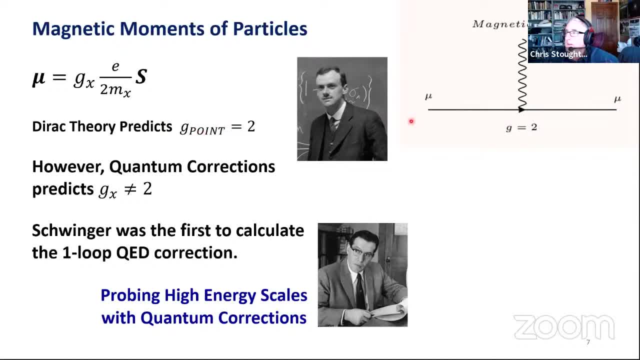 gyromagnetic ratio. So this would be, in casting it in Feynman diagram terms, right, The muon just goes right through, interacts at one point. the strength corresponds to a G factor of two. Life is simple, right. However, quantum corrections predict that. 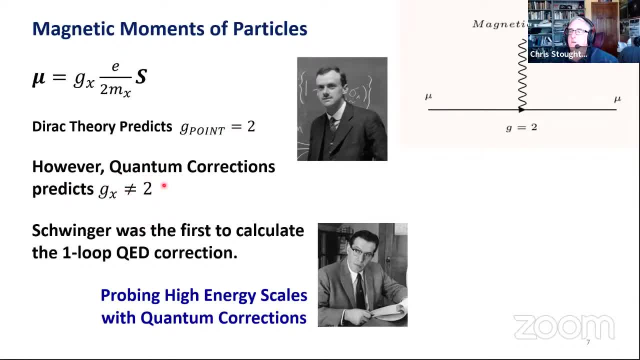 in general, the measured gyromagnetic ratio will be not equal to two, And indeed Schwinger was the first to calculate the one-loop QED correction right. And here is the so-called virtual photon taking a shortcut along the way, changing the effective strength all the way long of the overall 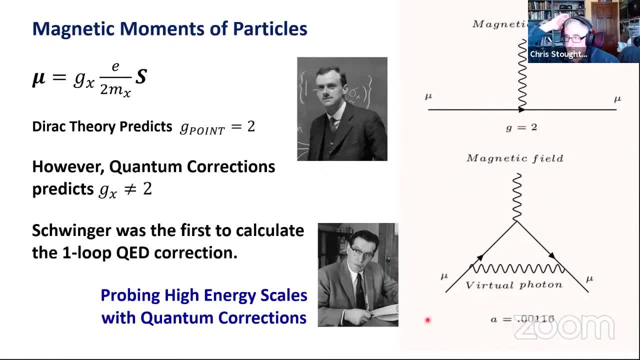 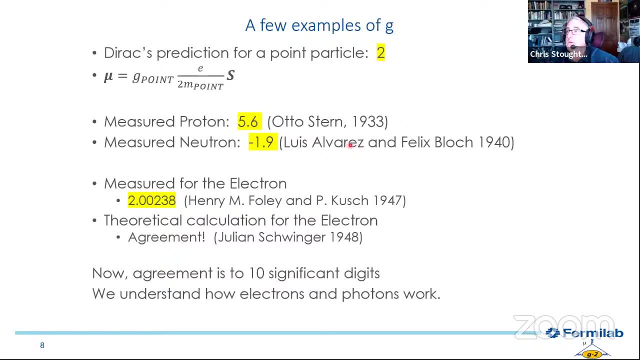 reaction and with this value of 00116, which is, of course. So this is a way to probe high energy scales with quantum corrections. So how did that work out? Dirac made the prediction that you should get two right, So let's measure it for a few things right. 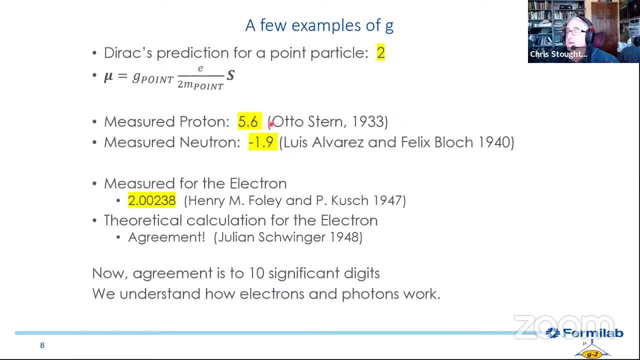 For a proton. Alain Stern measured it to be 5.6,. right Now some of us would say that's a lot different than two. I've had some phenomenologists say: well, six is about equal to two. So on some. 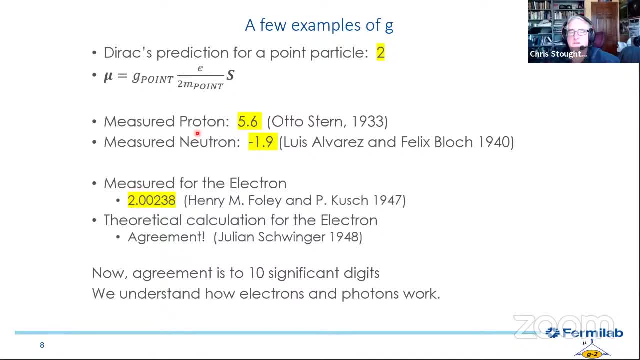 scales, there's general agreement. A proton is pretty much like a simple particle. Kind of more fun, the great measurement of Alvarez right And Felix Bloch, of Bloch's sphere fame, which we talked about all the time, went ahead and measured it to be negative 1.9. So even though it's neutral, 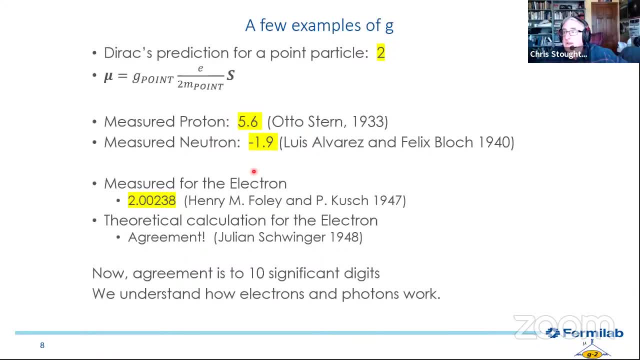 it should have no magnetic moment. Yeah, it should have no magnetic moment, but there's a combination of positive and negative forces inside the neutron which in fact give rise to its spinning backwards. right, This kind of is the first clue to what elementary students you know. 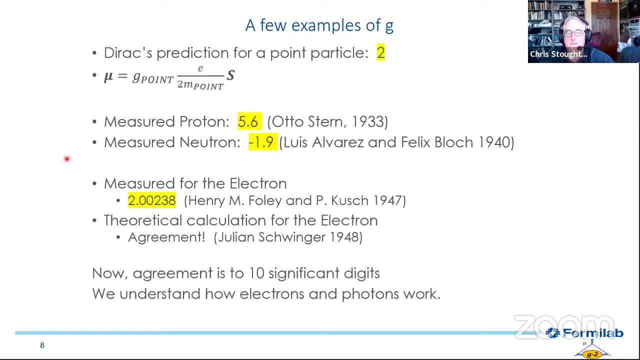 learned that you know protons and neutrons aren't point particles. They may end up with quarks and gluons, right? It's sort of common science sense. now to the people who have been indoctrinated in the ways of particle physics. The next precise measurement was made. 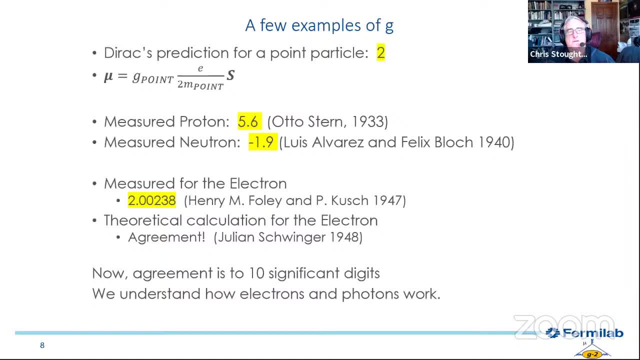 by Hohle and Krush in 1947.. I had the great honor to learn E&M from Professor Henry Foley of Columbia University right Now. this was, of course, well after his surprising measurement of g for the electron, And here we're getting closer. 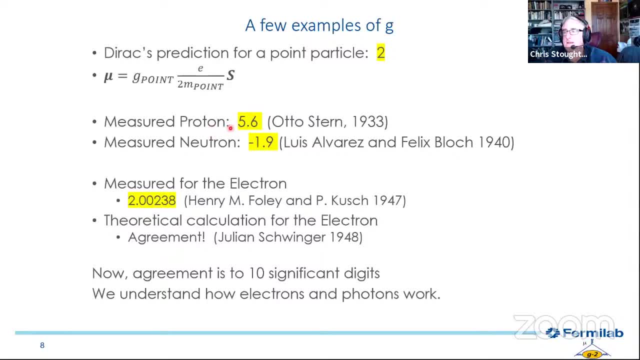 And I think people had started to come to terms with the fact that, yeah, the proton and neutron are so heavy they've got to be made of stuff, But by gum the electron. if that's not simple, what are we going to do? And it took about a year- six months to a year- for Schwinger to do that. 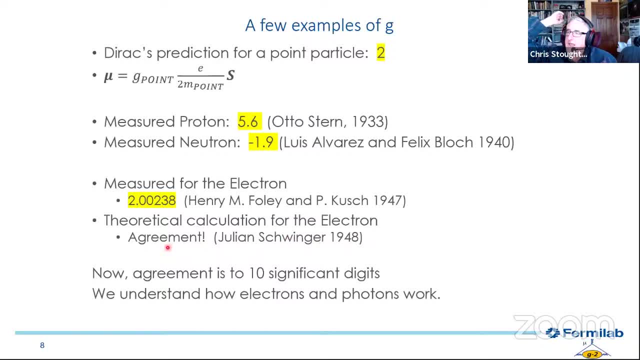 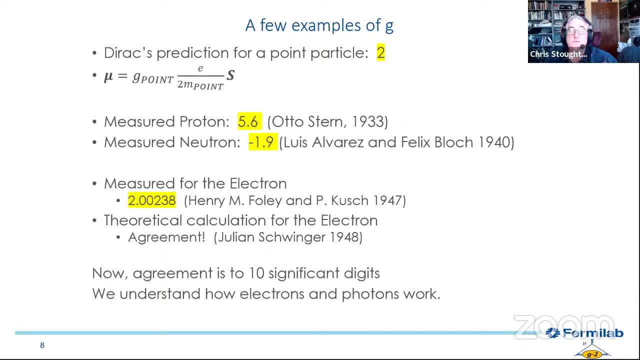 What turned out to be quantum electrodynamics, that, immersed in a sort of dynamic sea of virtual particles, Point particles get a little more fuzzy, Simple particles get a little more complicated And that's going to change the g value ever so slightly. So if people say gee, 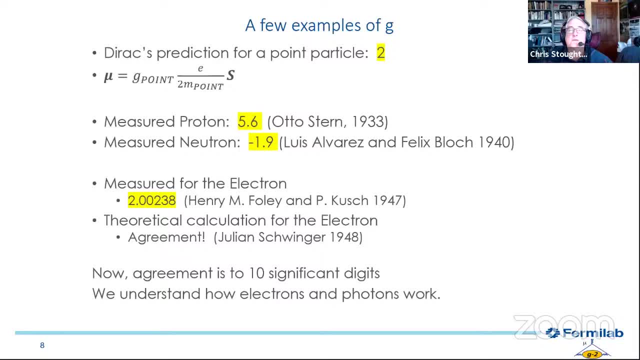 all this stuff with virtual particles you can't see, doesn't make sense. Yeah, but you can see an effect And indeed the modern agreement between the measurement, prediction of the magnetic moment of the electron is outstanding. It's similar to measuring the distance to the Moon to an inch and a half or something, And this is a case where the mysterious 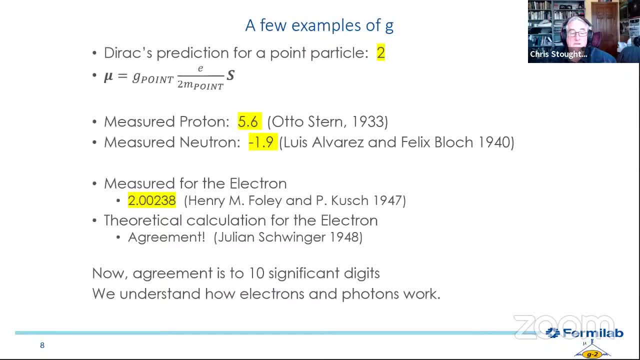 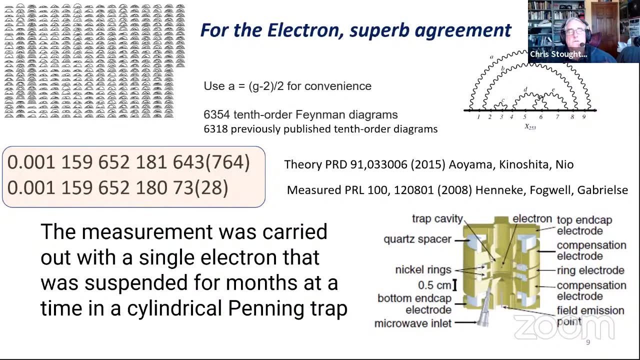 magnetism is perfectly explained by theoretical calculations. And let me take a side detour to just to- I don't know- revel in the glory of that experiment for a minute. I mean, if you write out these digits, it's always fun with when students get an answer on their calculator and give you all. 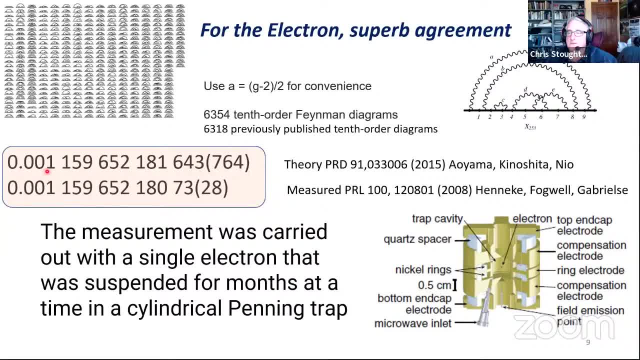 the significant digits. You have to explain about significance, But in this case it really matters. I really like writing these numbers on top of each other, right? And the digits just keep on getting the same answer all the way out here to about 10 significant digits, right? This is the measure. 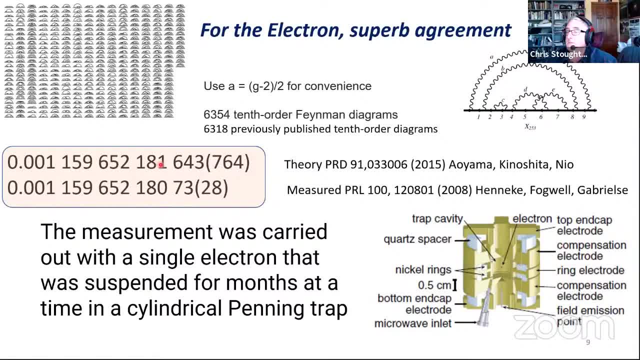 this is the theoretical calculation of what the magnetic moment of the electron should be be, And this is the measurement made by Gabi Alessi and others at Harvard. He's now doing great stuff at Northwestern now And so of all the Feynman diagrams, they'll make you calculate. 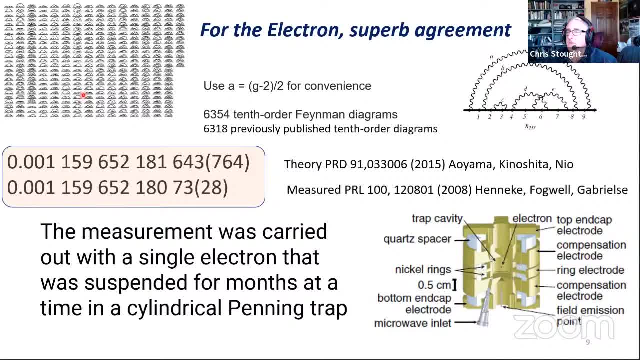 right. You've got to add them up right. First of all, you have to write down all the diagrams, calculate each one, add them up right, Put the phases right. This is just an example of one of the phases And there is ample homework assignments for graduate students to do to check this. 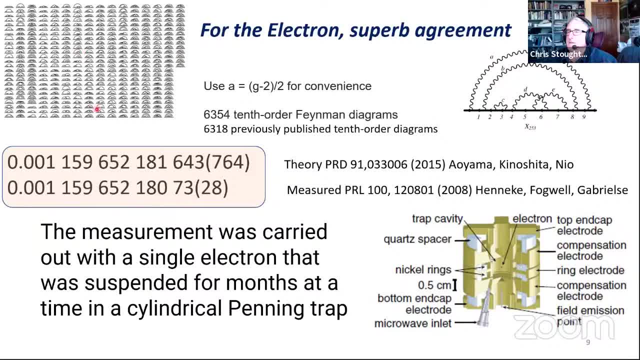 calculation In addition to the. you know the amazement of this calculation and this whole idea that there can be a varying bubbling sea of virtual particles is confirmed by this simple measurement. The measurement is its own triumph. You trap electrons and keep them suspended for a 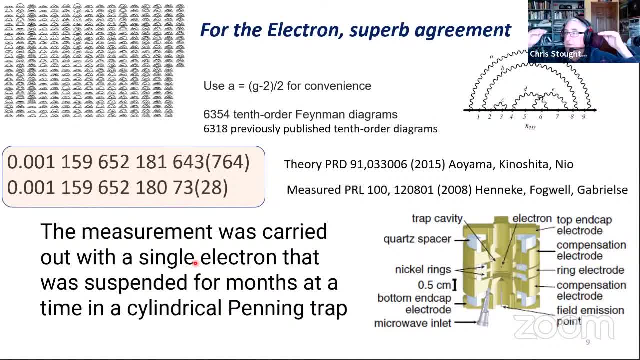 month at a time, suddenly changing their energy levels and then pinning right And, just you know, by dint of statistics coming up, And so you have to come up with your with the precision that you need to do. So it was in 2008,. 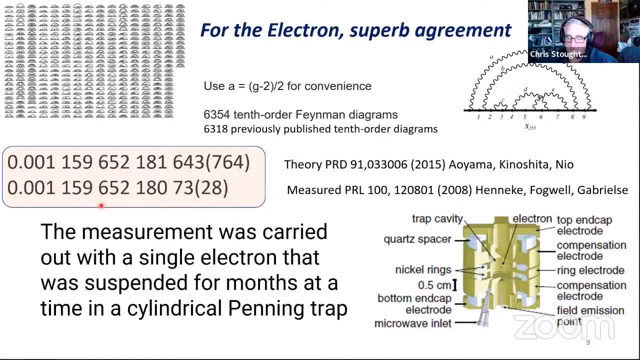 this measurement between 2015.. So it's a relatively recent measurement, And if anybody knows of any measurement physical science that agrees with a prediction to that precision, I'd love to hear about it. I can't, you know, we have measured other things more carefully, but the agreement. 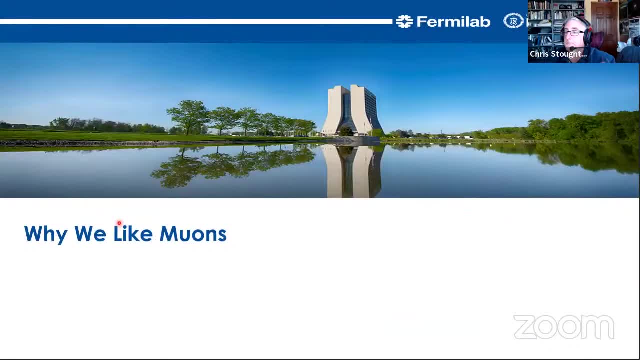 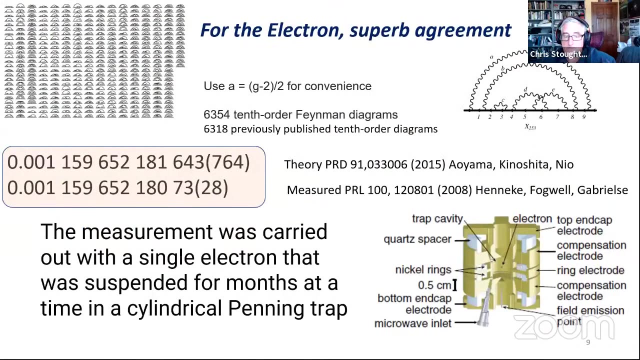 between measurement and theory is outstanding. Okay, So what's the deal with muon, Chris? there's a question: How do you get uncertainty in the theoretical predictions? Is the upper bound of the contribution of the truncated diagrams or something? It is to me one of the great mysteries of life of how theorists assign errors to their 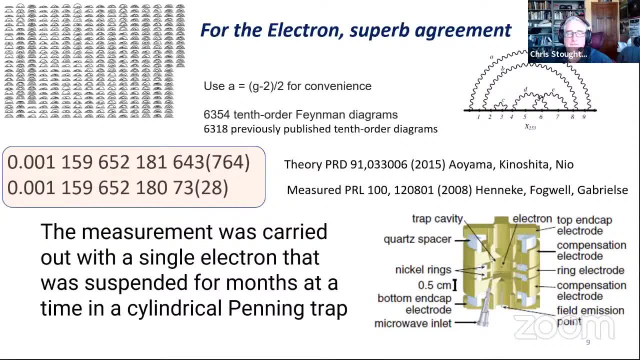 calculations. You know, when I do math I either get the right answer or the wrong answer. Now, some of it is: they take, you know, experimental data into consideration and then use that Other times your theories regard. use do Monte Carlo calculations to come up with other effects. right, But I'm well. 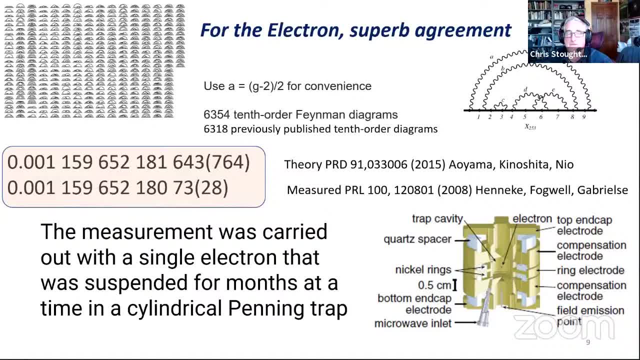 I can barely calculate one Schringer diagram, the Schringer diagram myself. I think that one's the exact calculation, And the actual guts of what goes on inside of this calculation is way beyond my ability to give you a full appreciation of it. 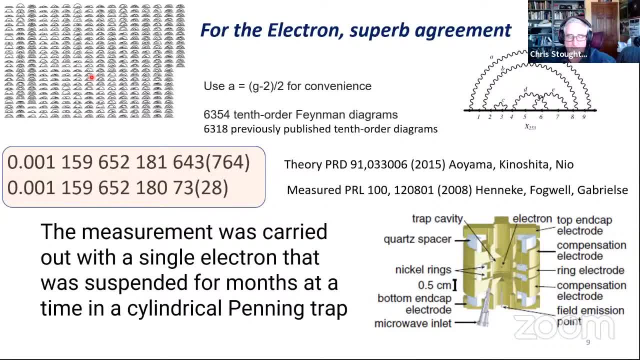 And it's even more fun when some theoretical calculations give you a statistical and a systematic error bar. I find that to be even more intriguing. But indeed there are. methods of calculations are limited And I don't think it's just merely truncating at six loops. 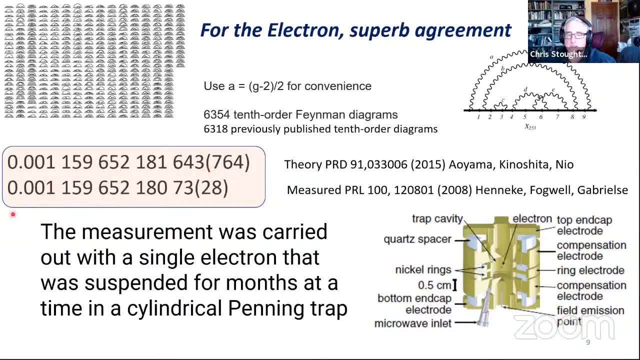 the five loops, And if there's a theorist who'd like to correct me on that, I'd love to hear it. And just sort of to presage that I've got enough trouble figuring out how experimentalists come up with an error question. 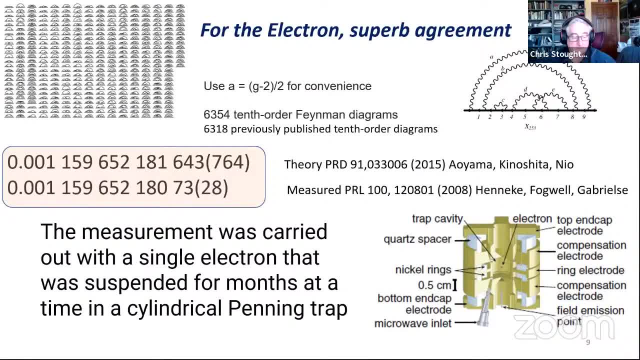 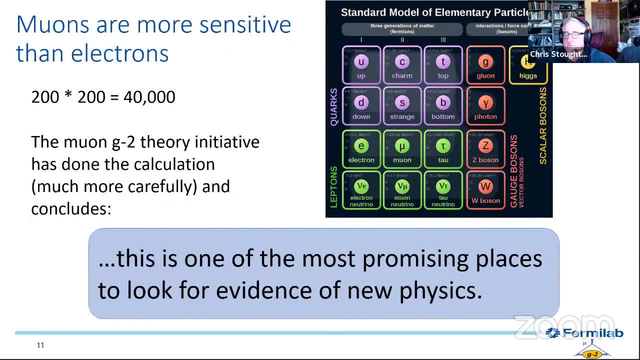 but that's a topic for later. I hope that addresses the question. I think that's great. thanks, Professor. Okay, thanks, Okay. so what's the big deal with muons? Why muons? Well, hopefully you've all seen the standard model. 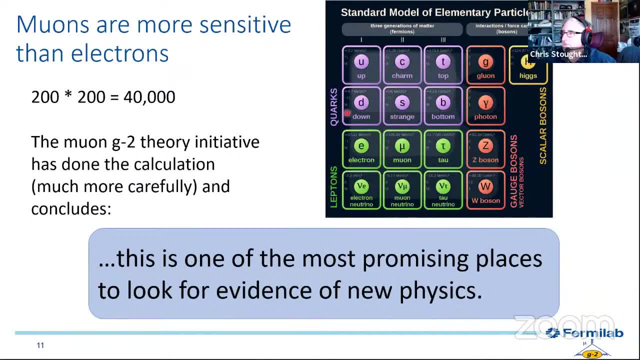 of particle physics. Right here is our periodic table analogy, just like you have for the atomic elements. So you know, normal people just worry about up and down quarks and electrons. This makes up the protons and neutrons. The electrons makes all of the elements. 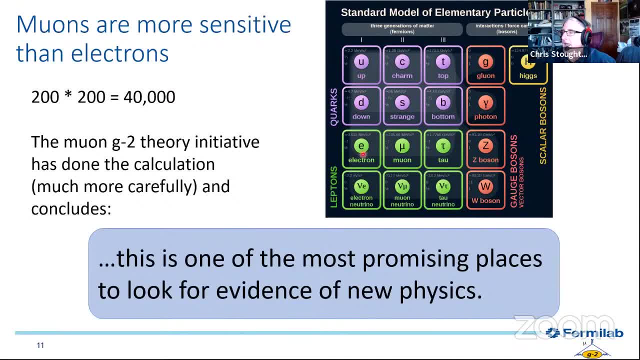 that we eat and drink every day, right. And there's four force carriers that we deal with. And for the electron, the calculation of that, it turns out, depends mostly on interactions with the photons: quantum electrodynamics. a little bit of a contribution to the weak forces, right? 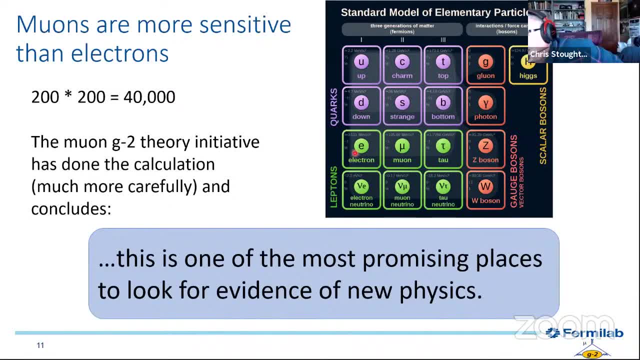 And that's the calculation that was done- to tensing the temperatures, The contributions from the rest of the standard model, in particular the quarks, the gluons, right And well, the strength of the weak forces is stronger too. scales as the mass. 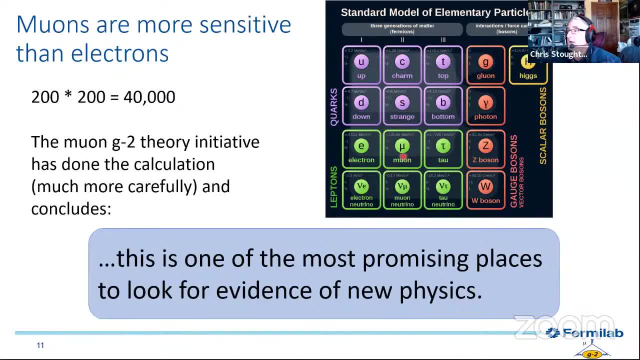 And since the mass of the muon is about 200 times the mass of the electron and it goes as mass squared, this calculation I can do: 200 times 200 is 40,000. This is 40,000 times more sensitive. 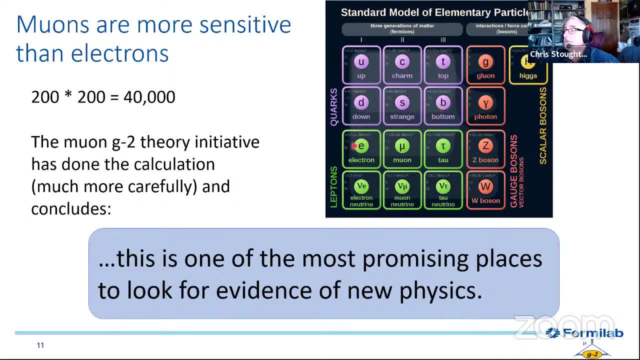 to all the so-called hadronic effects, right? So this is why it makes, that's why it makes such a great experimental probe. It is measuring the things we really want to measure, And indeed the white paper pointed out, you know. 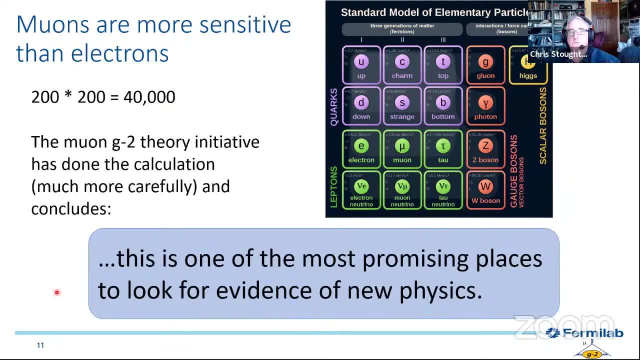 pointed out, this is one of the most promising places to look for evidence of new physics, because we've looked for evidence of new physics in well decay rates- branching ratios, creation of new particles- and it's kind of hard to see anything new. you can argue that neutrino masses are a clue that there's something new going on, but the bread and butter of physics- 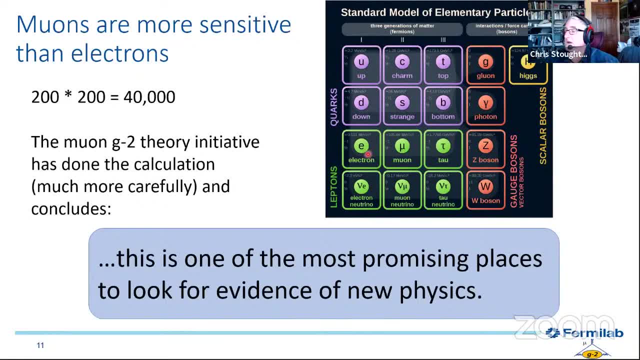 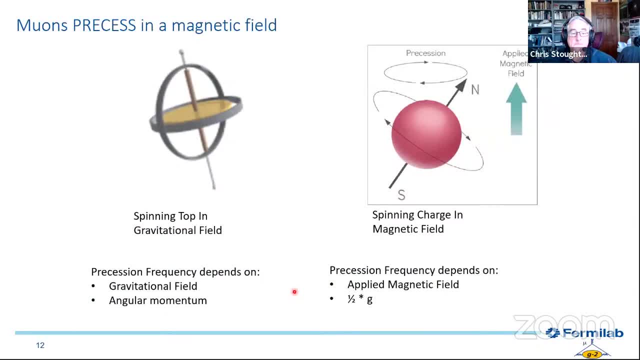 is what are all these strong interactions with? and this is the most promising place to look for evidence of new physics? um, of course, the other thing we like about muon is that it's kind of easy to measure this precession right and just as the top precesses in a gravitational field. 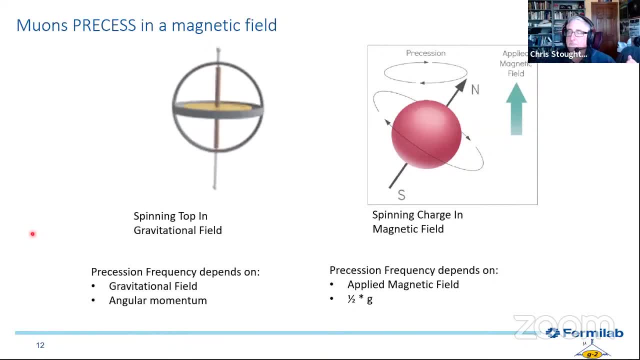 and its period of precession. we've all done this right. and just as the top precesses in a gravitational field and its period of precession, no more problem depends on the strength of g, little g, um and um the angular momentum. how fast you're spinning the top, um, uh, that will uh tell you. well, measure two of those things you. 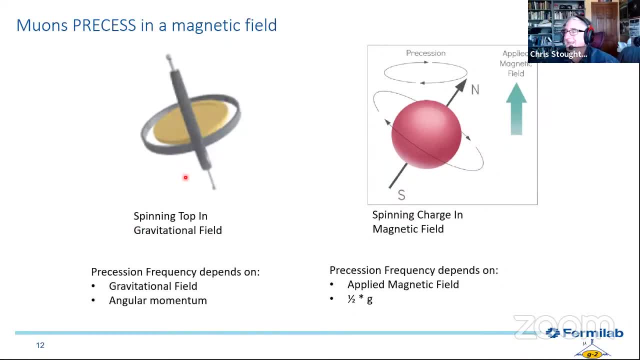 know what the third one is, so you can use that in any of those three ways. in an analogous way, a spinning charge in a magnetic field will also precess, and that precession frequency depends on how strong is the magnetic field you're applying right and how fast is that thing spinning. what's? 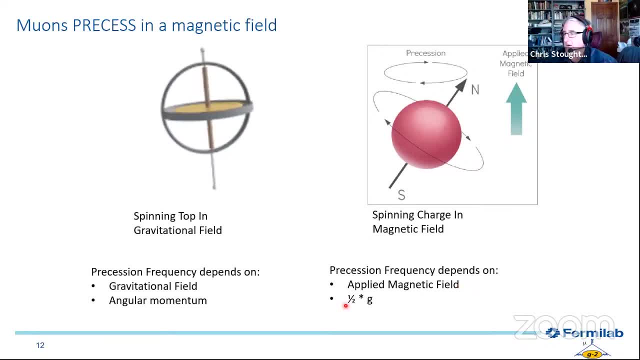 its angular momentum right, and for our units um that's one amplitude right. so analogously, it's the same experiment. if i had one muon i could put it in a magnetic field that was exactly one tesla if i could just watch it precess, measure how fast it's precessing. i do the experiment now, of course. 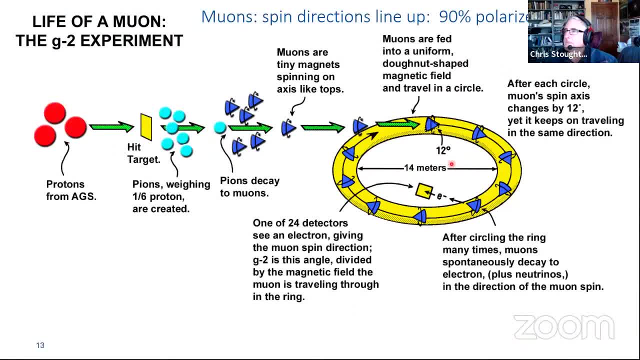 you can't do the experiment quite that way. you can't do the experiment quite that way, um, so um, you have to use some very fortuitous properties of muon. it turns out they are also amenable to do an experiment, which is quite convenient, right um this. this cartoon was. 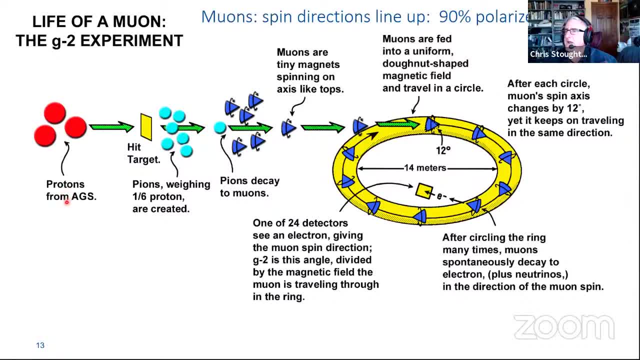 drawn for the brookhaven version experiment, but frankly we haven't been able to draw a better one, so just keep using that one here. the protons come from fermilab. you hit a target- mostly the stuff that comes out. anytime you hit protons in the target, you get lots of pions and 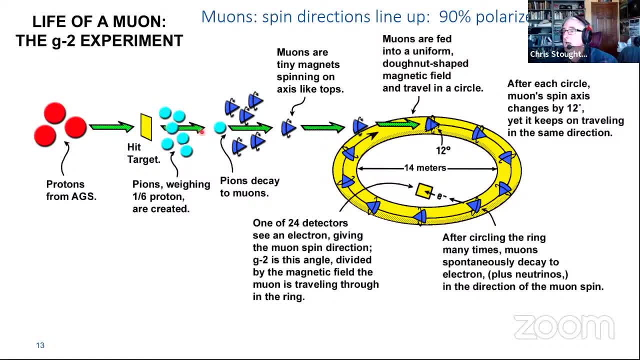 then a few other things. um, these pions after a while decay into muons which, lucky for us, are pointed with their spin, pretty much in the direction of the momentum. i mean, yeah, there's a distribution, but there's a very strong correlation to, uh, the direction the muon is going and it's 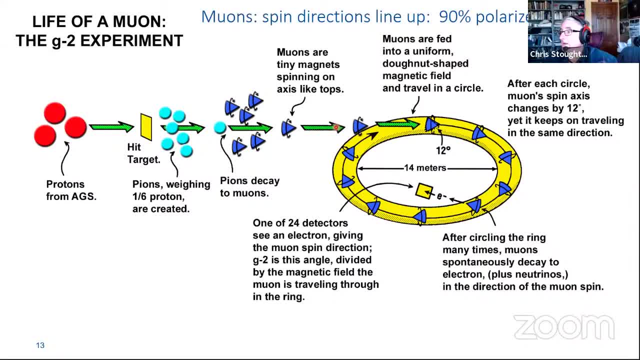 spin, and then somehow i'll tell you that later. you sneak these guys into a storage ring where they go around. the cyclical electron frequency makes them go around in a circle. that's easy, right. and then there's a little bit of precession happens too. if g was exactly equal to do to two, the spin would always. 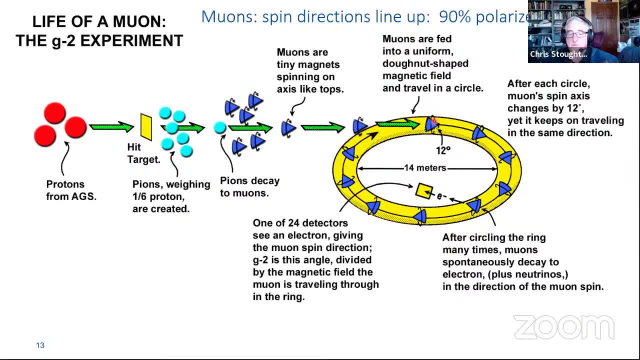 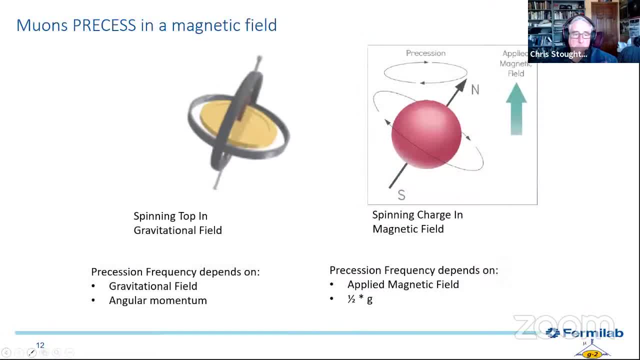 line up with momentum, but there's a little bit of excess precession, and that's what we're going to look for. so that's the other reason we really like muon, the first being is- i'll go back a couple slides- is they're very sensitive to the rest of this physics so we can look at. 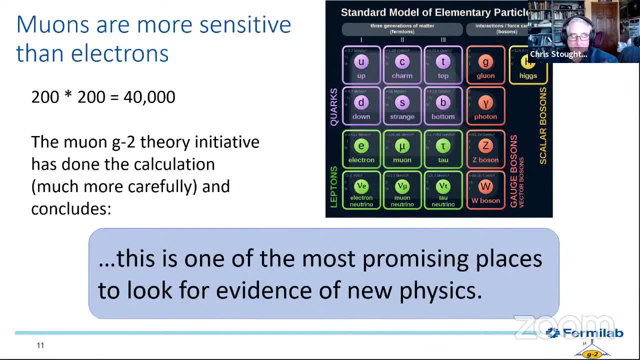 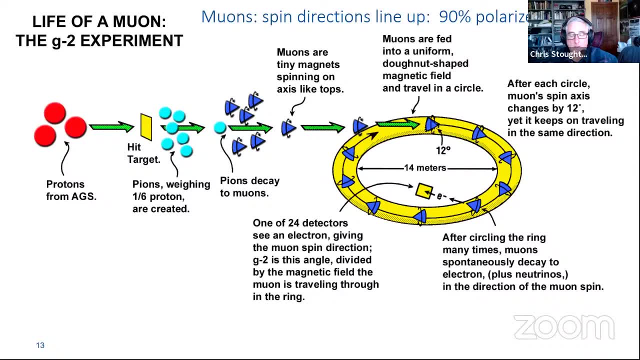 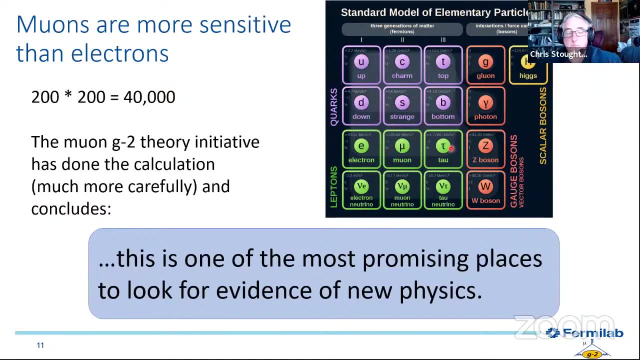 them a little bit more. and then the second is that they're just gosh darn convenient to make and store in a convenient way, right? um, i think if you were to be an extremist you'd say: oh great, you've done the electron and muon, now let's measure the magnetic moment at the tap. uh, and 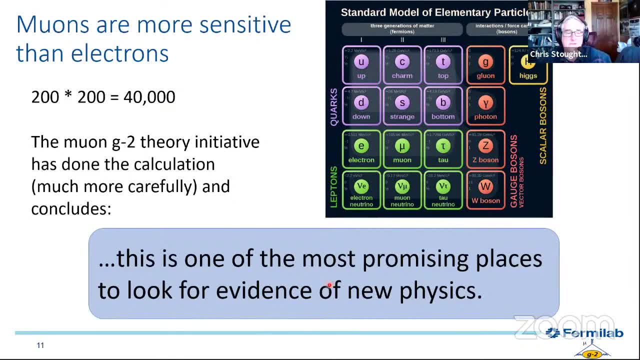 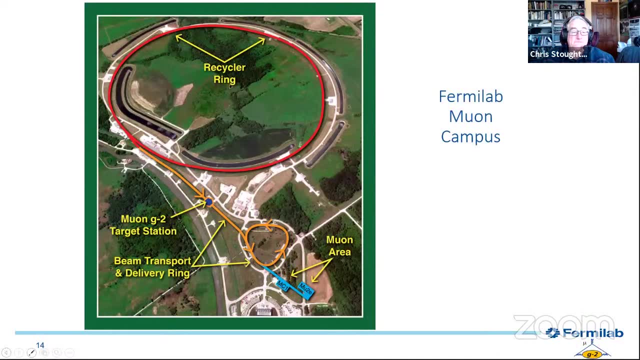 you'll be um saddened to learn how short its lifetime is. and if you can figure out a way to do that experiment, um, let us know. okay, here's a view of what things look like at fermilab. uh, the accelerated protons hit the target, so we get the recycler, um, and then the protons hit our station here. 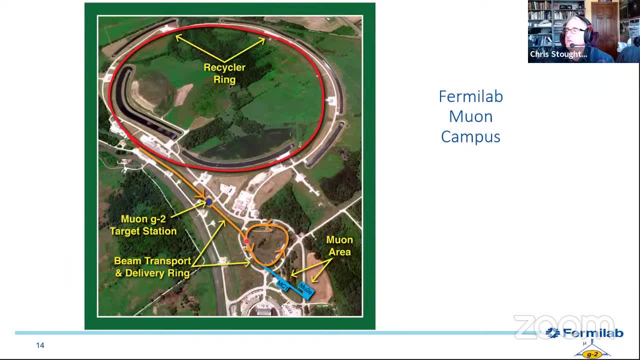 right, and one advantage we have over brookhaven is we have this little storage ring, what we call the delivery ring. um, some of you old timers will call it the uh anti-proton source. it's the. it's where we would store the anti-protons for the. 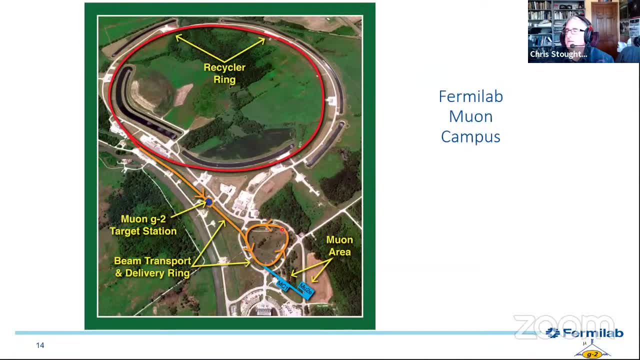 tevatron, right um, but it's been repurposed now to be delivery delivery ring. you go around it depends three or four times. that gives a chance for most of the pions to decay away and then you can eject in a pretty pure beam of muons into the uh, accelerate into our um, into our experiment. 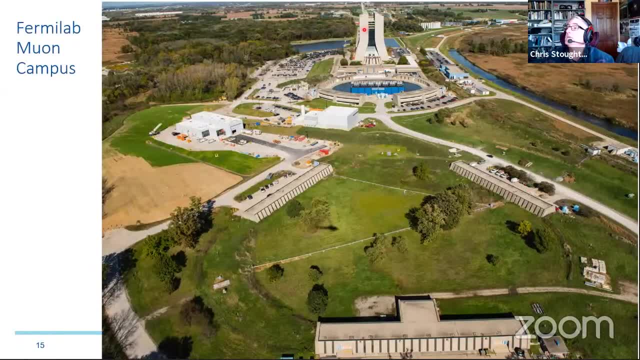 right. here's another picture now, looking at the backyard. so, but the buffalo are way out here. this is wilson hall. if you look out the backyard of wilson hall, here is the anti-proton source, and just let me tell a story about john peoples, who built the anti-proton source after he was director. 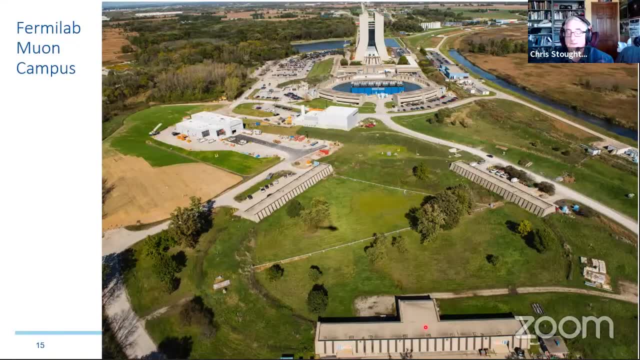 he loved coming back to visit the lab. he would sit and talk to people and some of the some of the postdocs on g-2 were explaining to this guy right what they were doing, and there's this delivery ring with lifting. so he was very patiently listening to them and saying okay, thank you. and after he left i said: 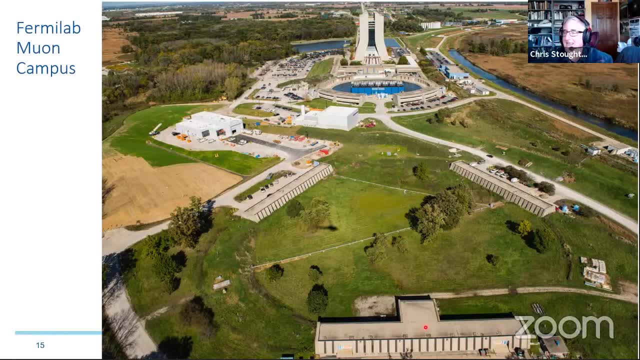 do you know who that was? no, that was john people. so what did he do? he built that storage ring you were just talking about, except he called it the anti-prognosis. john was very gracious that way, okay, so anyway. so they came around here and then, uh, this is our experimental hall. so if 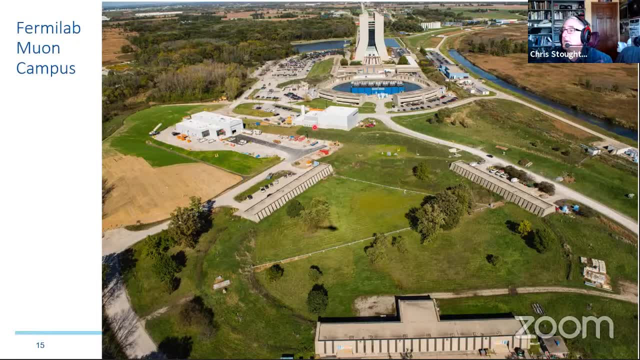 you ever get to visit fermilab again, drive around the back and come out and visit us. the other experiment that is coming online is the is the mu2e. we're looking for direct conversion of muons to electrons, um to a even more rare process. 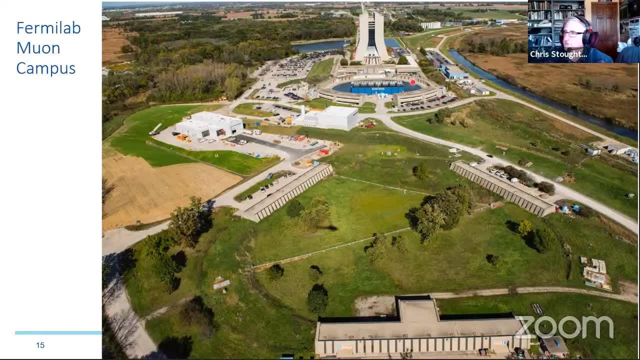 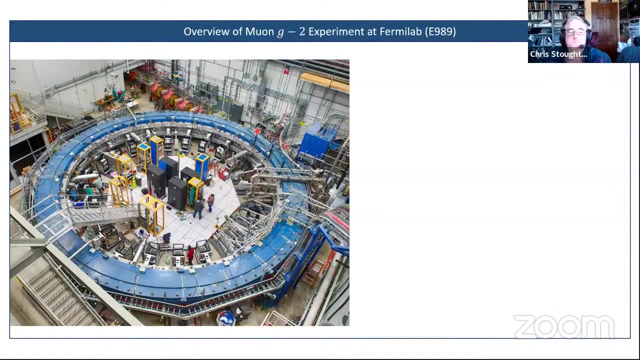 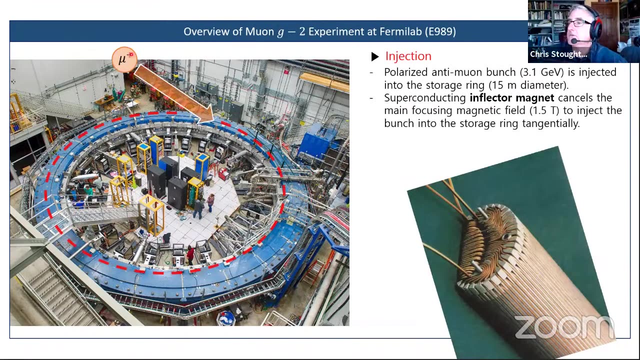 and they're going to be sharing and eventually taking over the muon base for us. so they're over the ground and that's in the middle of where we are. okay, good, okay. so let's do the experiment. the muons come in right from the source up there and this is flipped around backwards much more. 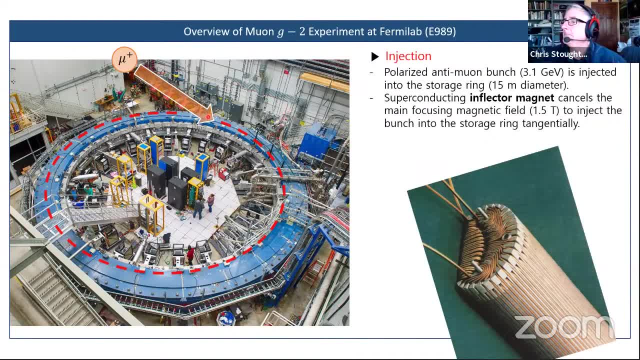 we're seeing before. sorry about that, and um, of course, the problem with the magnetic storage ring is, if you have a charged particle coming in, as soon as it starts seeing the field it's going to bend and hit the wall right. so you have to drill a hole in your magnet and put in a so-called 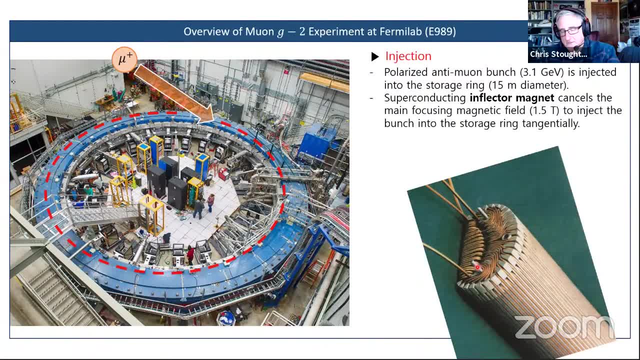 inflector magnet which has a magnetic field in the opposite direction. so the muon sees no field until it gets all the way inside of the ring right, and then it comes out the end of this and says, oh, there's a magnetic field. i'm going to go around in a circle, so that's how you get. 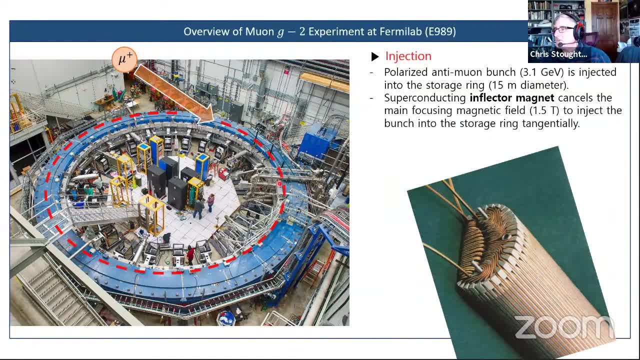 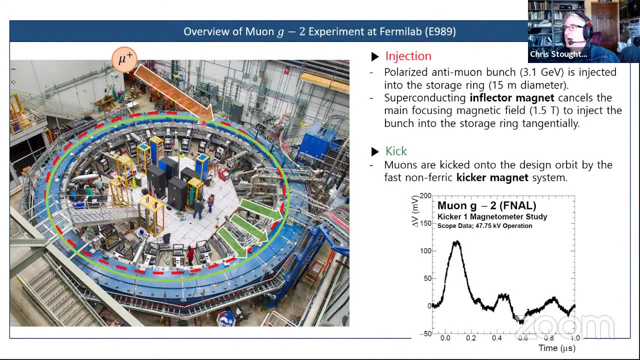 uh, the muons into the ring. if that's all you did, they would go around one time and then hit the inject inflector again and you'd be done right. so you got to do something else. that's where the kicker comes in. that's the thing i worked on. right is um right after. 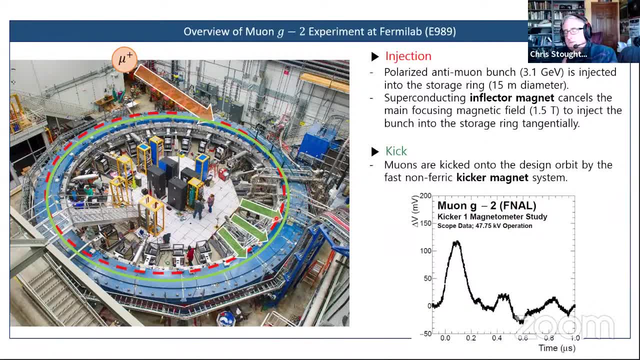 they come in. you have long plates that form an electromagnet and you pulse it with the field that makes you do it the right way. um, that reduces the magnetic field so they don't bend as much and you can see, see, here that's sort of like a hula hoop- changes that red ring around to the 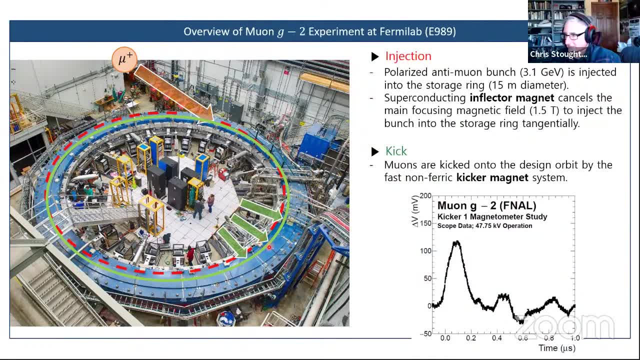 green ring. so after getting that kick here, the muons will go around and then miss the inflector and then be on a stable order, right? so this is the voltage as a function of time that we kick with. it takes a little bit longer, right? so it's about 100 microseconds. 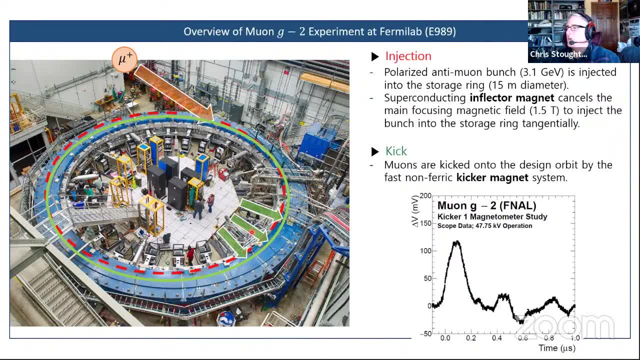 to: um, i'm sorry, 150 nanoseconds for the muons go around one time, right. so while they're going around, the first time you get kicked and uh, i'll just tell you now. the problems we had were a couple. one is the kick wasn't strong enough and two, it had these after kicks and negative kicks. 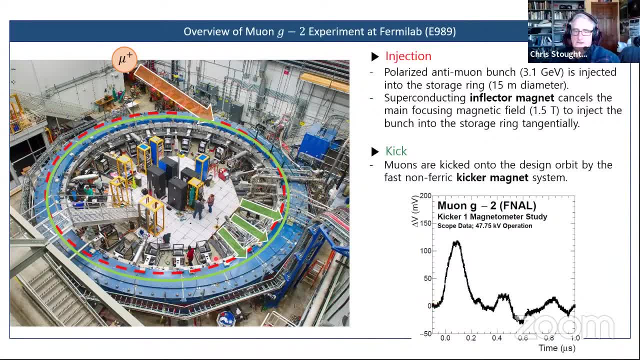 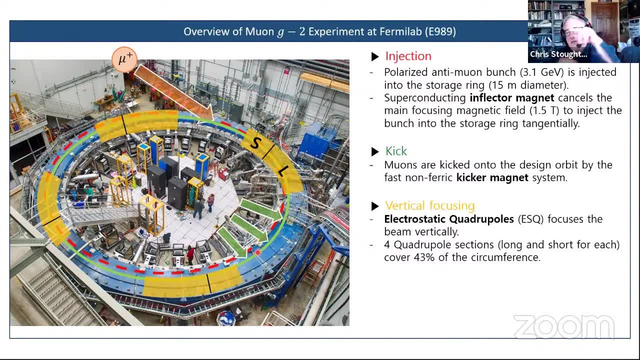 that messed up the game. we're sort of fixing this okay. now the next problem you have is that if you've got an orbit that's not going exactly straight, if it's going a little bit up, it'll just keep spiraling up and hit the ceiling, or spiraling down and hit 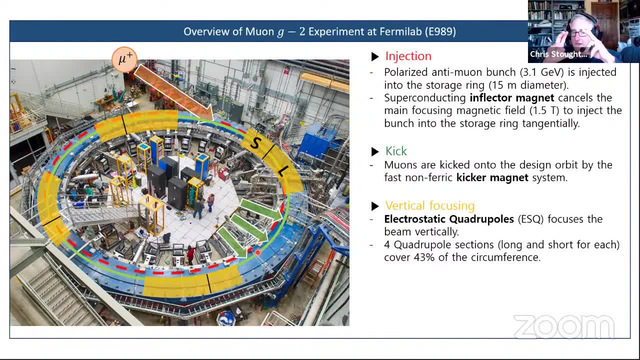 the floor. so you have to have focusers in there. quadruple fields, the electrostatic field, quadruples. um, that will. you know, particles that are going up will push down, particles that are too low will push up. so at least you will then have stable orders and this gives you the ability to store the 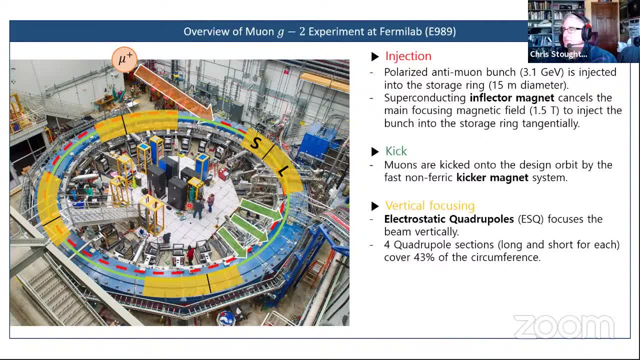 for you know thousands of of orbits, long enough before most of the muons. um. the problem is going to come back and bite you, though, is because a relativistic particle going past that electric field will see it as a magnetic field, right, and that will also call precession. so you're going. 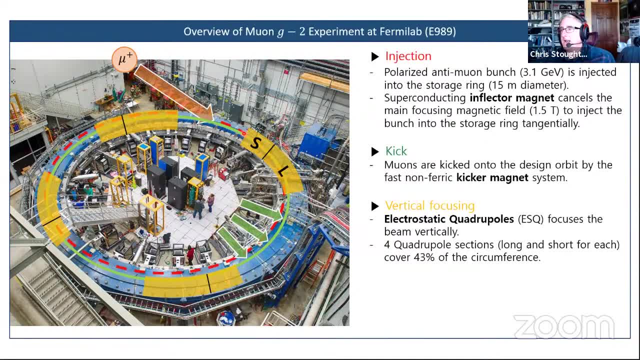 to need to know the amplitude of that electric field to the accuracy you're going to know the magnetic field, and that's really hard to do. so there's a trick we use for that, which also right. finally, we've got the muon stored and we wait for them to decay. uh, lucky for us, right? 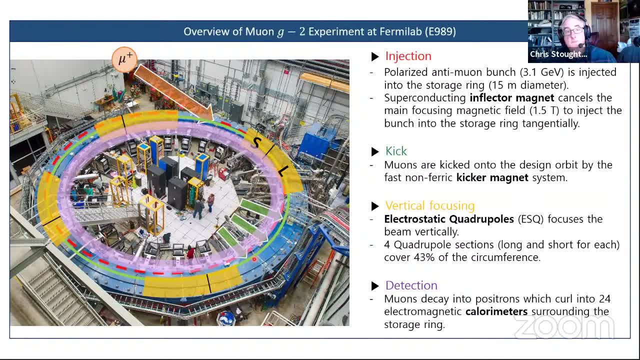 muons. not only are they born in a convenient way, but they decay in a convenient way. that is, when i'm a muon and i decay, um, my positron is going to be sent out, where the momentum of the positron is correlated with the direction of my spin. so you can ask which way was that muon spin pointing when it decayed? 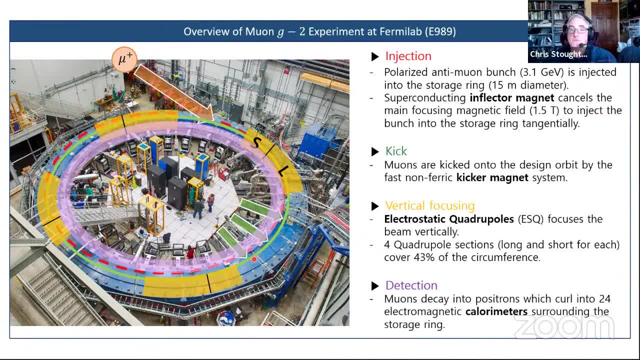 by answering the question: which way was the positron right? so, um, an electron's of less mass, so they'll curl in. so all the way around the inside, at 24 stations in fact, you can see them here. here are the calorimeters that see little tiny showers. every time a positive. 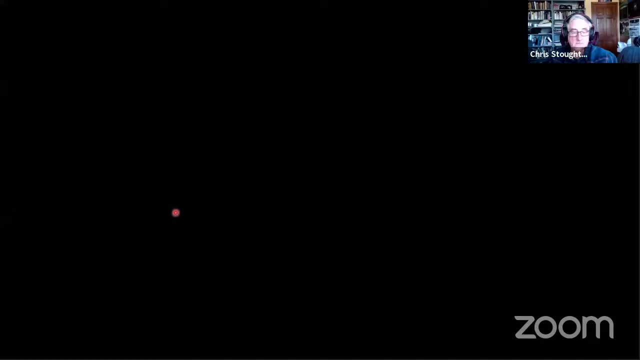 and if i can figure out how to start this, you'll see a video. okay, half the time i do this presentation, it works and it doesn't wait. here we go. so this is a video of what immune seasons it goes around the ring. here's a simulation, so this is awesome. 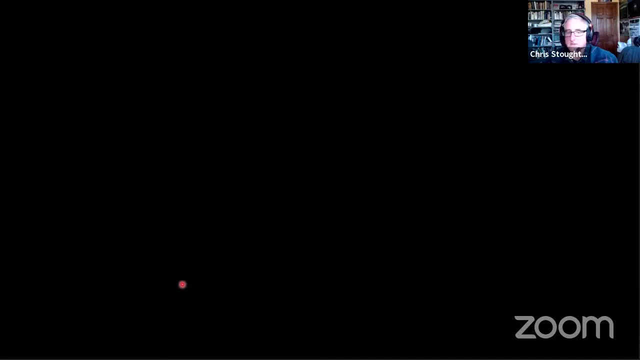 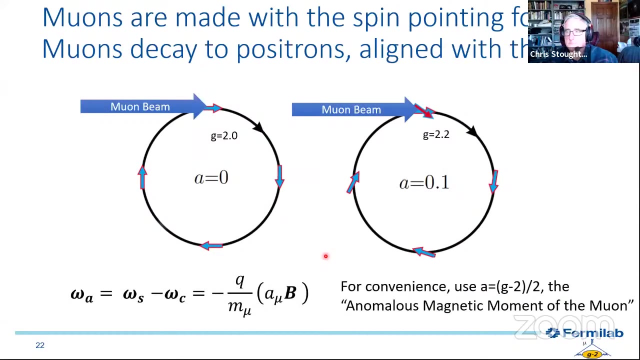 all right, so let's talk about this. we're going to go throw the muons right to the right side now and this is a part of their co-creation process. you can actually use the muon and also the muon. the muon is the co-creation process. we're going to show you. one minute here how important that is when you take the muon to the right side and you're able to see these co-creation patterns that are上下断, MA2, and you can see that they are not normal. but we have some of that and they are normal and i'm going to show you how to do this to them. 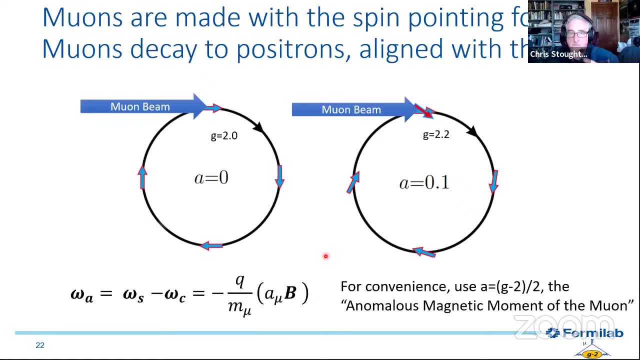 are because, obviously, when we go back and do the simulations, we do full j on simulations to right to simulate what our acceptance is as a function of time and position. okay, let's move on. as i talked about um, if g was exactly equal to two, the momentum and the spin, 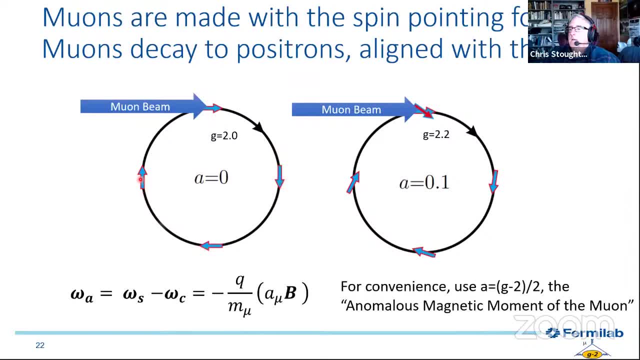 would always be collinear and one preset. one cyclotron frequency would be one precession frequency and this would be like the moon, you always see the same side of the moon here. um, what really happens when g is a little bit bigger than two is, as you're going, you can. 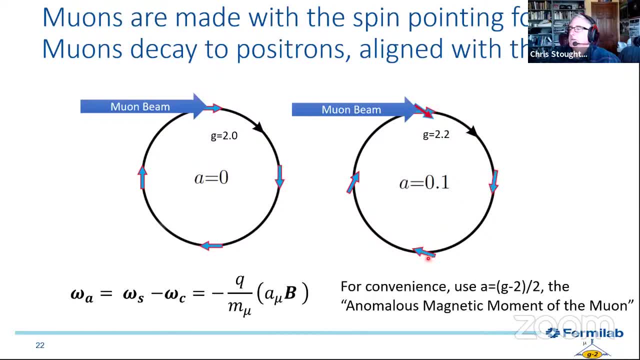 see, here the spin is pointing a little bit more in. here the spin's a little bit pointing more in. here the spin's pointing a little bit more in. and it's precisely this difference in um, the cyclotron and the precession frequency that we measure, and convenience to make the math work. 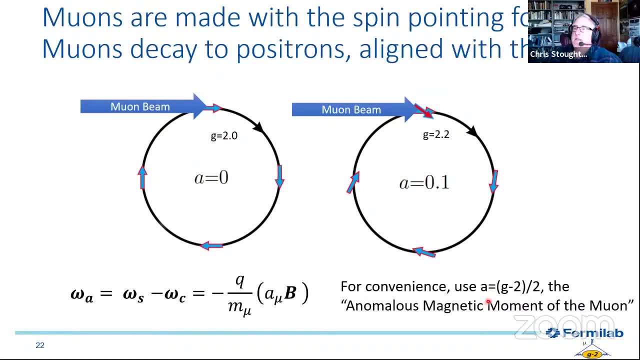 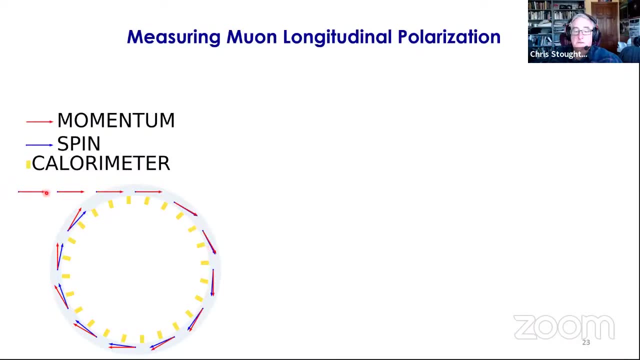 out easier. we use this a as the anomalous magnetic moment normalizes g minus two over two. that's just going to make the algebra later. um, and here's a more detailed look at the process: the red arrow is always the momentum which way the muon is going. um, see that around the ring. 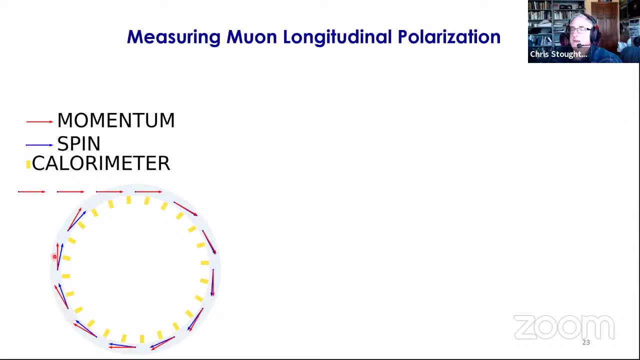 it always points straight ahead. the red is always pointing straight ahead as it goes around the right. doesn't look like it here, but but it is right. the blue area arrow is the spin direction at each point. so you can see here they're on top of each other. all you see is the dot of the blue going here, and even after you go a little bit you. 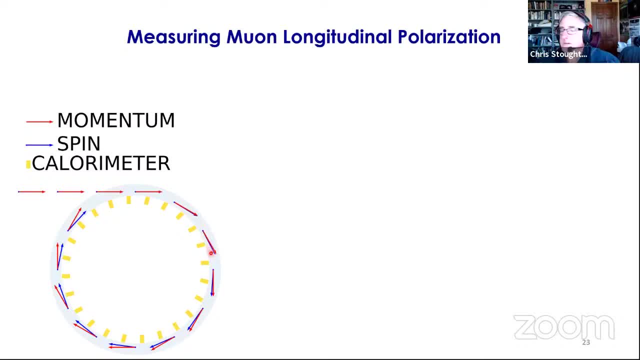 see the little bit of concession the blue is pointing a little bit more, a little bit more here, a little bit more here, a little bit more here. then, when a muon decays: when a muon decays, wait a second, ah yes. when a muon decays right in the center of mass, right, the spin um. 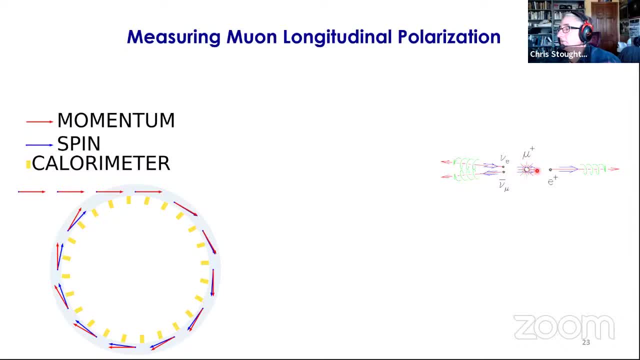 parity is conserved. so, um, you know, the positron goes in the direction of the muon spin right, where the blue and the red here line up here, blue being the spin right and, uh, red being the momentum. of course, in the center of mass you have no momentum, by the way, neutrinos go the other. 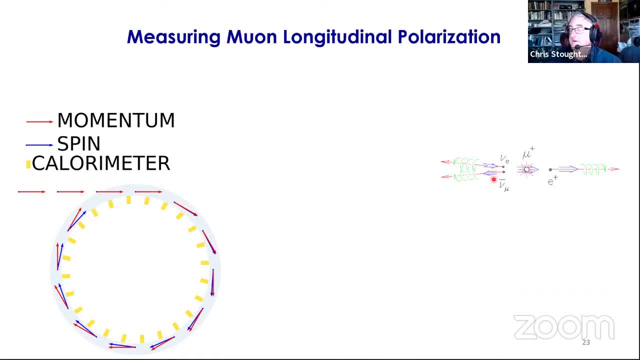 way- and yes, this is a way- to go to the center of mass. you have no momentum. you have no momentum. wonderful neutrino source, very monochromatic, um. so you talk to your neutrino friends at fermilab and do some calculations and realize you'll see like one neutrino event every 10 years. 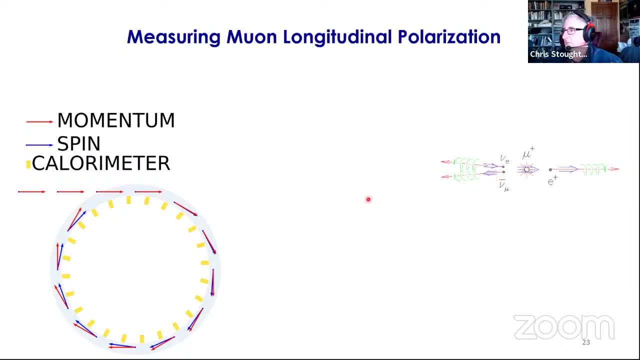 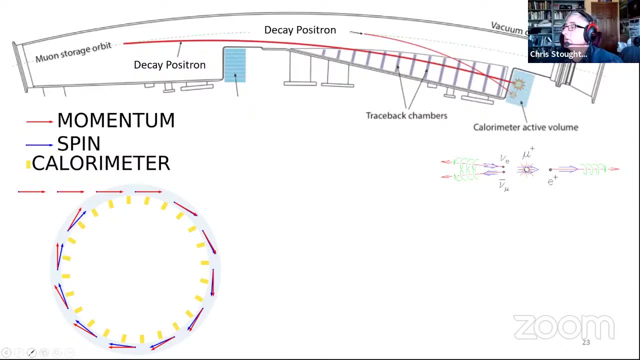 in their detectors are so incredibly pathetic. small numbers, so not practical as an IT source. but it's monochromatic. if you then boost to the lab frame it looks like this right. so this decay right happens. let's say it happens here. when the spin was lined up with the 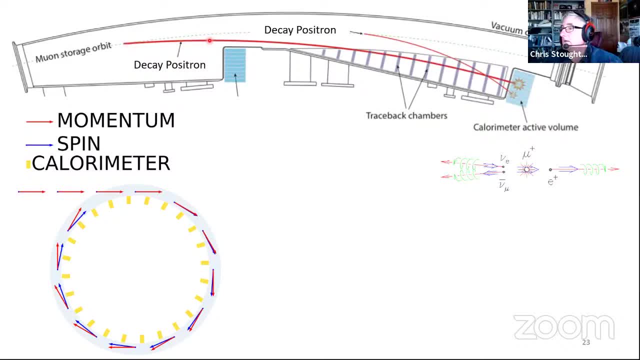 momentum. then you boost that electron positron momentum. it's got a lot of momentum and it goes and gives you a nice big splash right in your calorimeter. we also have tracker chambers to decalibrate. um, if it happened here and you just happen to be in a moment when the the spin and 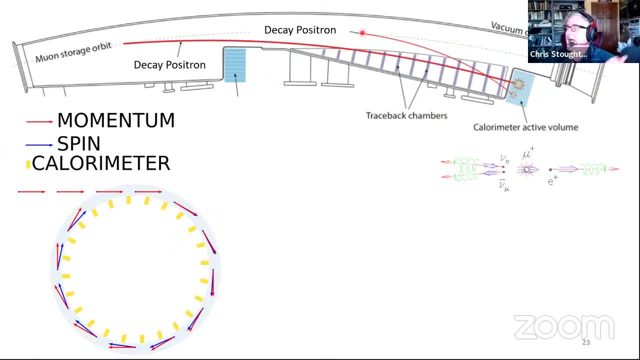 the momentum were pointing in opposite directions. well, you're going to not have as much momentum on that positron. it's going to have a lot lower energy. it'll curve faster and, of course, give you less energy in the calorimeter. so that's what you're really making now. if you decayed in this. 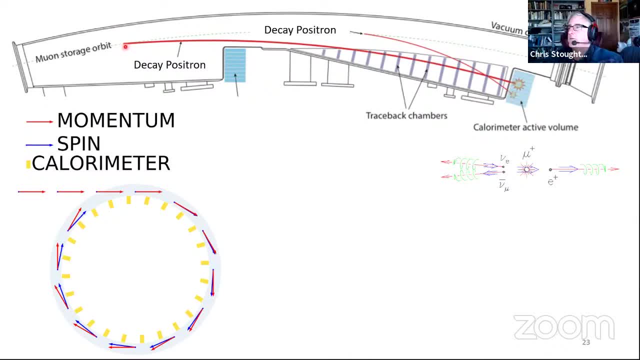 position and your spin was pointing in the wrong direction. well then, you would just hit the wall. so we don't have a hundred percent acceptance. but these are two examples of events that wind up nicely in our calorimeter, coming from two different positions. um, that helps describe what we're doing, right. so there are 24 places around the ring where we make that. 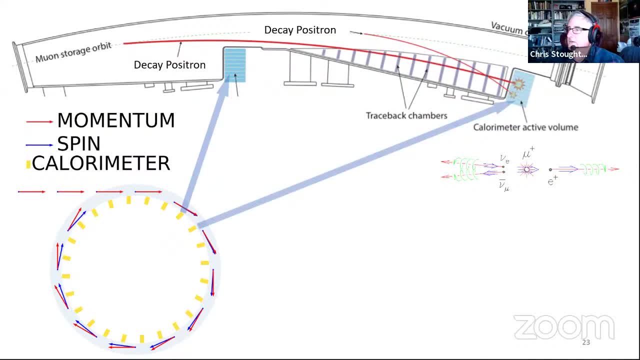 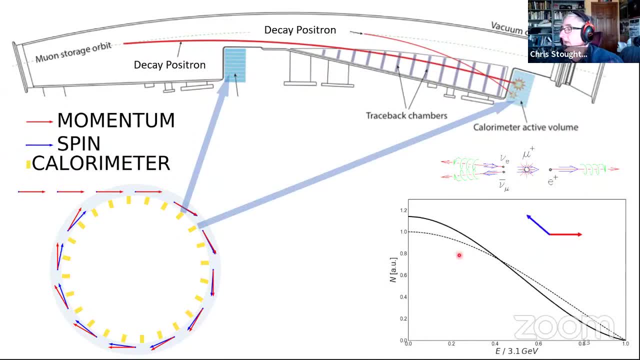 go as and as procession happens, right the spectrum, you measure, right the number of events. um, as a function of energy, um changes with a characteristic frequency, and that's the frequency we're looking for, that's the procession frequency we're looking for, right, um, and one way to think about doing the experiment. 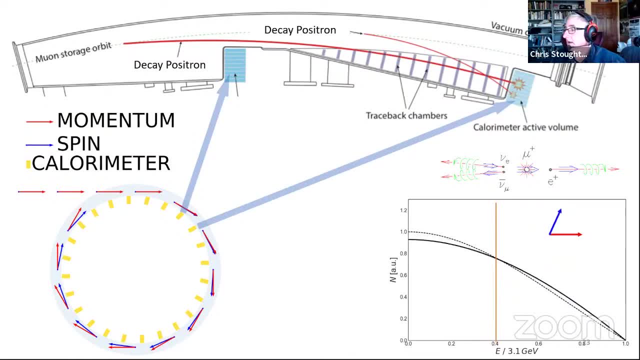 is to say: well, i'm just going to put a threshold there right and just count the number of events. and as I count those number of events, I'll have more and less, and more and less. and there are other ways of doing the analysis. you can ratio what's the number I have? 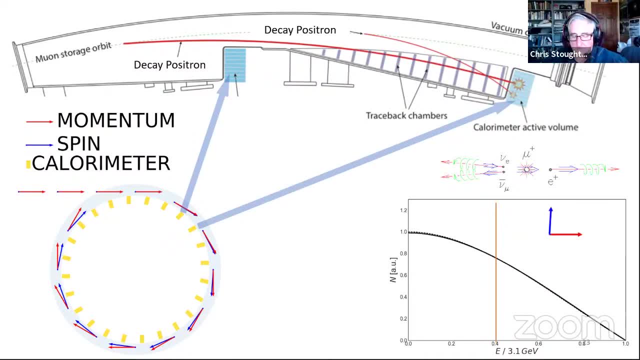 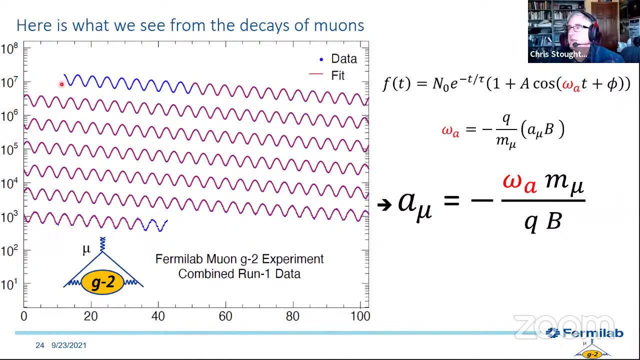 left and to the right. you can fit the distribution lots of different ways, and indeed the analyses have done it many different ways to get there right. okay, so that's how you wind up with what we call the so-called wiggle plot. you see here, going electric. 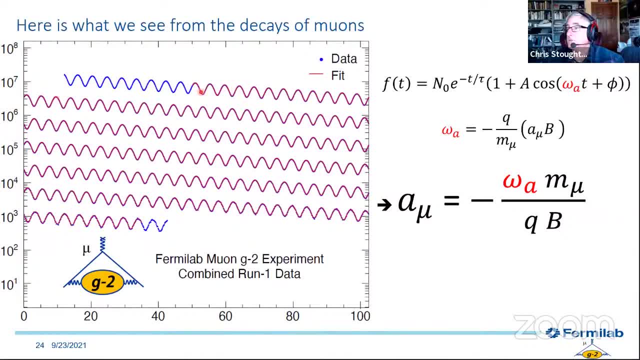 left to right, top to bottom. this basic trend is the lifetime of the muon right. as you go along, you have fewer and fewer counts, right, and here this up and down is the precession right, and if this is all we had, you would simply take the Fourier transform of this, find the peak. what that? 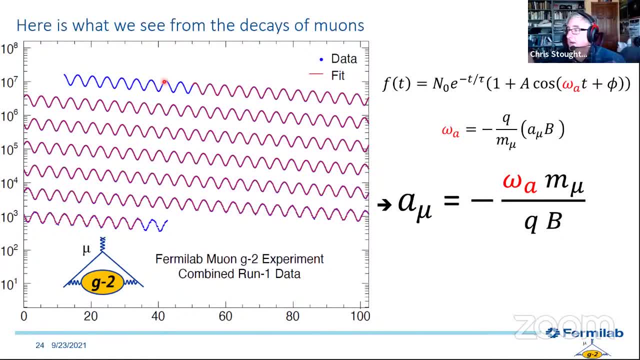 frequency is, and then you can take the Fourier transform of this, find the peak, what that frequency is, and you'd be done right. and then, since you know the mass of the muon and the strength of the magnetic field exactly, um, then you would calculate the anomalous magnetic moment of the muon. well um. 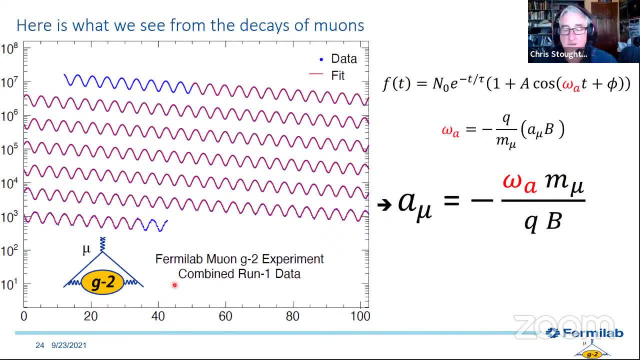 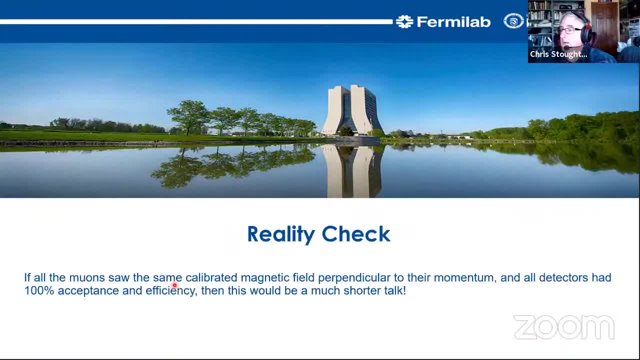 that's, in principle, how you could do it, but to get our kind of accuracy, uh, you've got to worry about now all of the fun stuff that you do first of all. um, well, so this is a reality check. so that that's the basis of what we're going to be doing in the next couple of years, and then we're going to 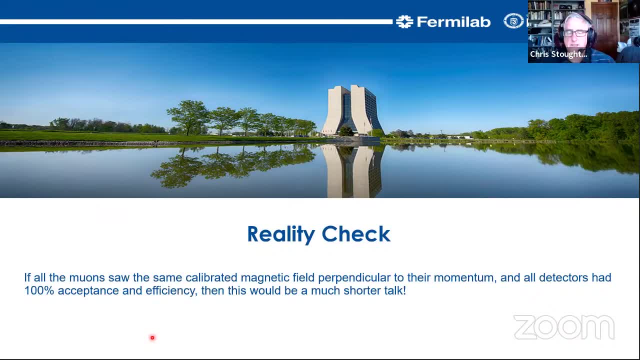 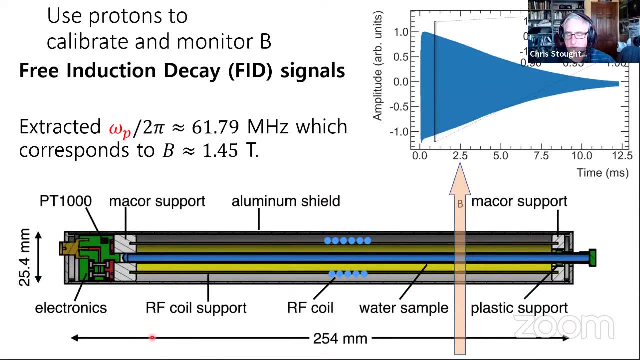 we're going to be doing in the next couple of years, and then we're going to strategy of the experiment. i hope that that works out for you. and now i'm going to dive into the gory detail. and the first is, of course, we don't know what the magnetic field is, and it's different. 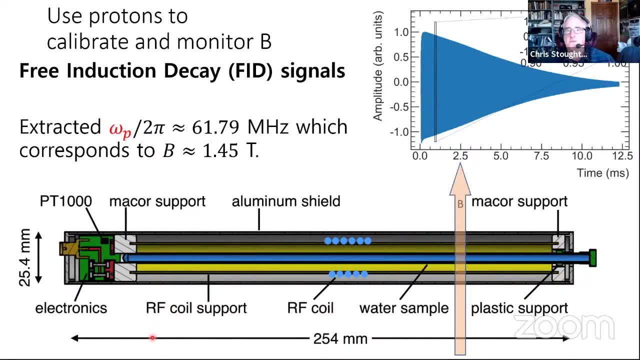 in different places inside the ring and it changes as a function of time. you know, someone opens the door and the hall heats up a little bit, the jaws open up a little bit and you change the magnetic field. so you're going to worry about stuff. so we're constantly monitoring. 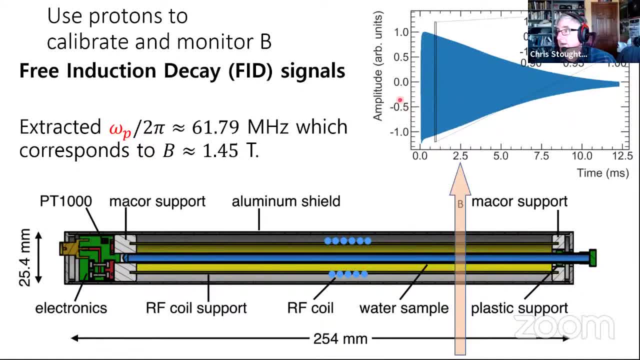 the magnetic field, um, using nuclear magnetic resonance with gizmos that look like this: this thing is about 10 inches long right and about an inch and well, it's, it's, it's an inch in diameter, uh, which we call 25.4 millimeters, uh, and it's got a sample of um water in here and you have a little. 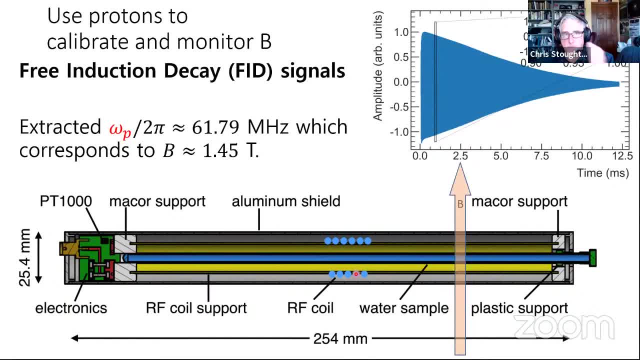 coil that i can send a pulse through. when i send a pulse through that, it's going to line up all of the protons to be going sideways. okay, now it's sitting in the static magnetic field that we're trying to measure, so those guys are going to start precessing. right, and they're going to precess and 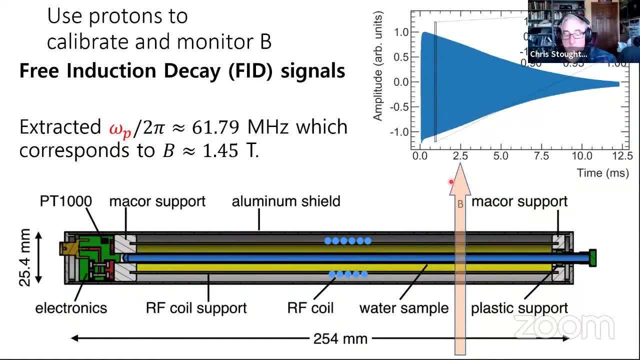 relax up so that they wind up pointing straight up. so as they, when you hit the pulse, they're precessing with a big signal. and as they're precessing around, you read back on the same coil. they're all radiating like a little antenna radiating right um, except they're all rotating. 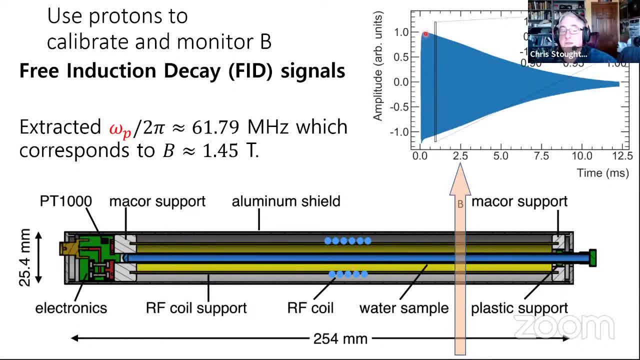 in the same direction here, um, and so you get a coherent signal pattern, and if you just zoom in on a little bit of it, you can see this frequency. this is the precession frequency of the proton, which depends on its magnetic moment. you're going to ask someone else what that value is. 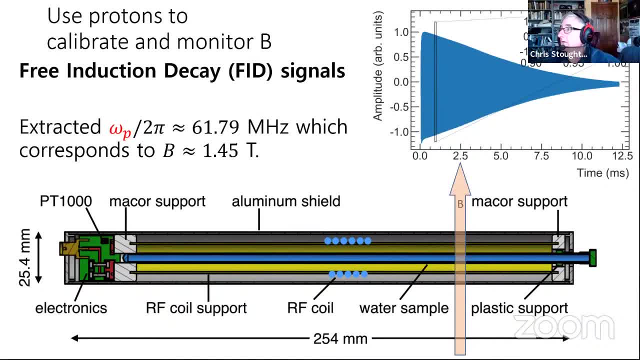 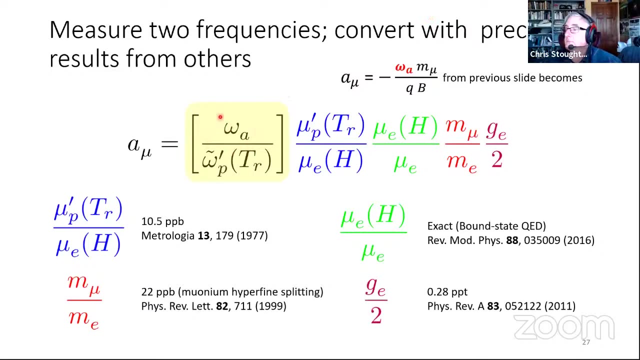 and the strength of the magnetic field. so by monitoring this proton frequency, we're constantly monitoring the magnetic field. that's the basic strategy and there's an entire paper on the magnetic field. okay, so we're going to do two things. we're going to measure the precession frequency of the muon. 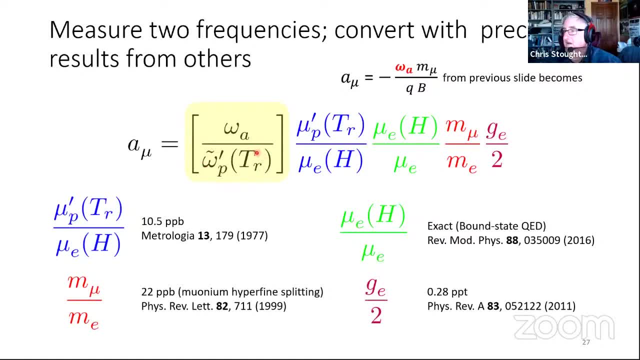 and then we're going to measure what the precession frequency of protons are for all that, where the, where the tilde, the dash and the temperature, um, all relate to things like what is the temperature of the thing is? is the shielded or unshielded? so we've got to get that all straight. but anyway this. 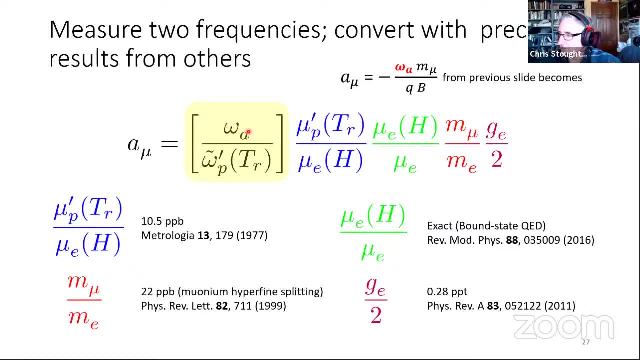 is the precession frequency of the muon, the precession frequency of the protons. you notice here now that the magnetic field has dropped out of the equation right, and you then sort of need to normalize that by two things. this first factor is the electron g factor in hydrogen. 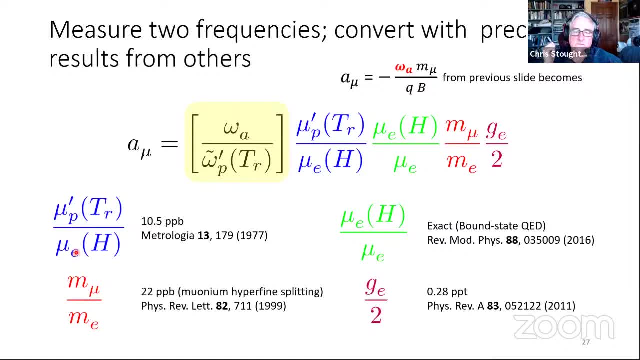 divided by the proton g factor, and this is in a sample of water, in a spherical sample of water. right well, it's the proton to electron. let's see you work it out that way. so this was measured very carefully back in 1977, which it's a standalone, beautiful experiment. 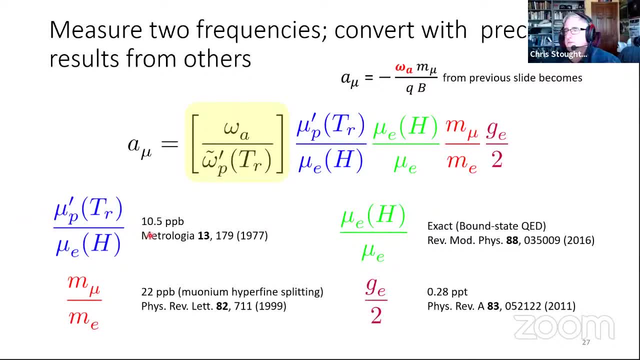 all by itself. um, nobody's done better since then. so we use this value and its precision is 10 parts per billion, right? i think this was done in mit and stanford, sorry, um, and then this number here is from muonium hyperfine splitting. you have to know precisely, like we all say, oh yeah, the. 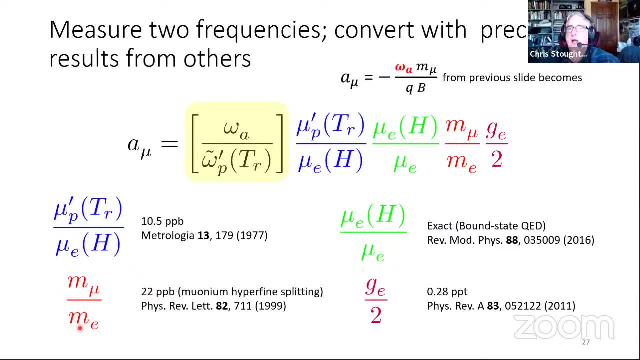 the mass of the muon to the electron is 200.. if you're high, if you're high precision, ah, it's really 211.. so 211 or 210, whatever right, but we need to know that. to 22 parts per billion. and it's another beautiful experiment. you make yourself some muonium. 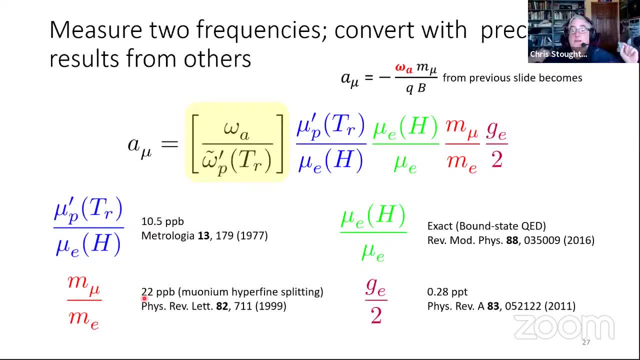 and get it in the ground state and then do the hyperfine splitting in a strong b field, right, so you can do a microwave magnetic resonance spectroscopy. um, i think you have to know the magnetic, i forget. no, i think you get from that directly. you get the, the, the mass ratio of the. 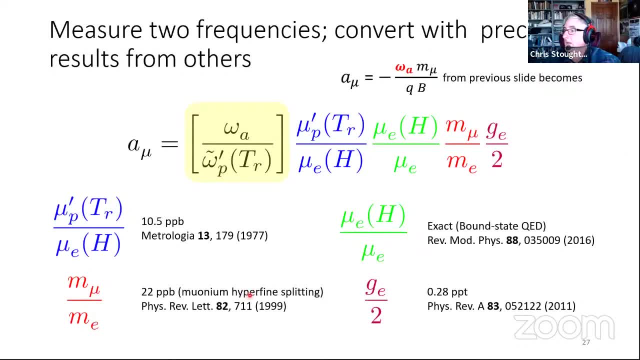 electron and that's the most precise measurement of that um. getting the magnetic moment of the electron right when it's bound to when it's free is an important correction you have to do, and this is a direct calculation. we got the latest value here from code data, their publication, um. 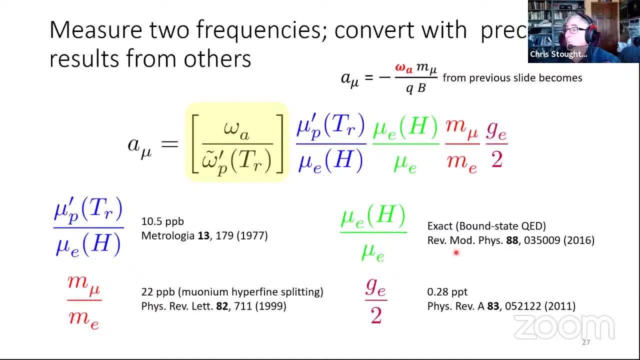 then of course it all depends on the magnetic moment of the electron, which we already measured in that other experiment. but then So there's 0.28 parts per trillion. I love quoting that here. So this is an exact calculation. This is less than a part per trillion. 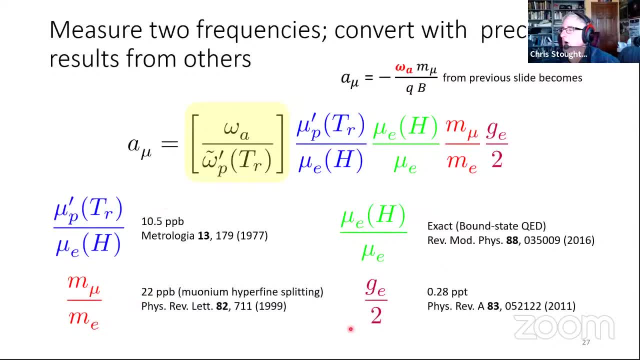 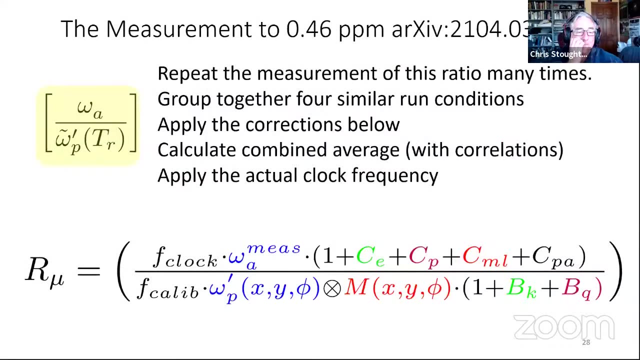 These are a few tens of parts per billion. So all of these external measurements contribute to the error of this ratio a lot less than our measure. Okay, so what do we do? Yeah, so to get this right, You don't just measure this one. 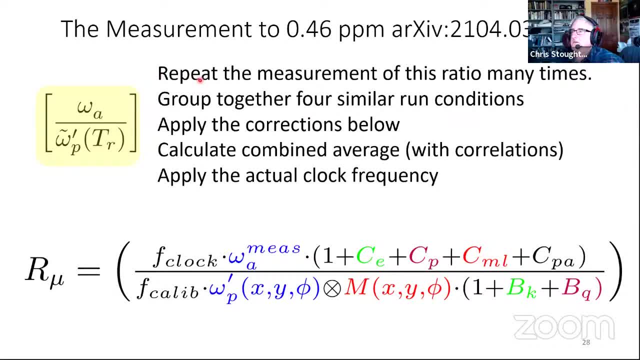 for one fill and be done right. You have to repeat this measurement many, many, many times to gather enough statistics for your statistical uncertainty to get small enough to be worth it, right. And then, since you can't always run an experiment the same way all the time, 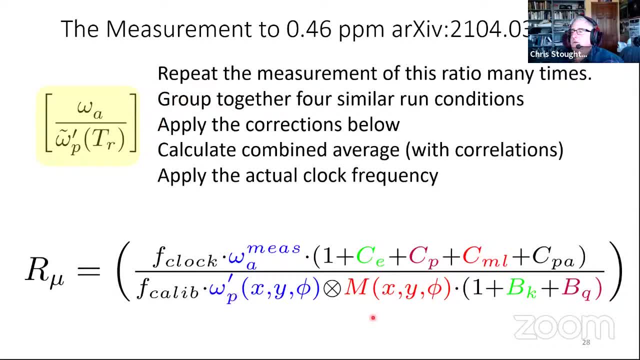 you group together similar run conditions And then there's a bunch of corrections we know we have to apply right. For example, the kicker afterwards leaves a little residual field. for a fraction of the time you're starting to use The quads leave a residual field. 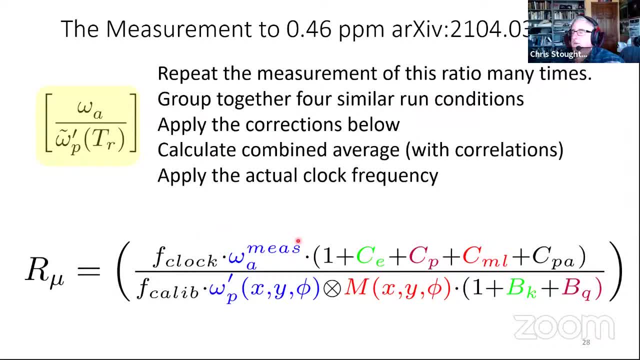 And right, there's many other measurements. So you measure these things and you also have to convolve what the actual magnetic field right, What the actual magnetic field is as a function of position in the ring and position inside the ring with where the muons are right. 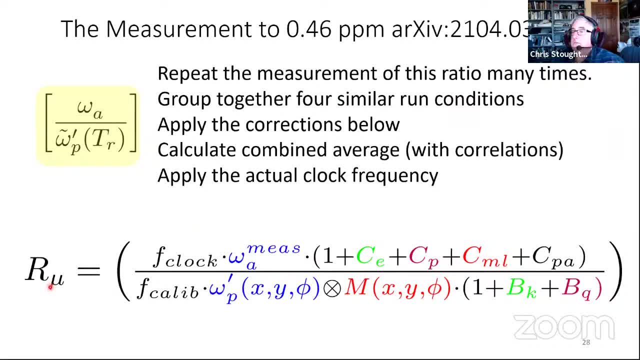 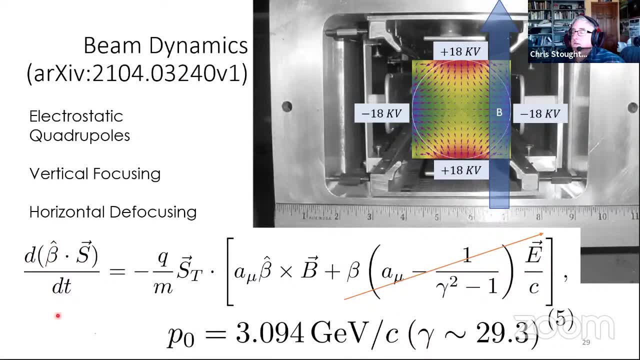 So that gets you your so-called R value. The other nice correction you can make is the precession frequency right Depends on the electric field you use And depending on the relativistic boost factor, it has this correction in front of it. 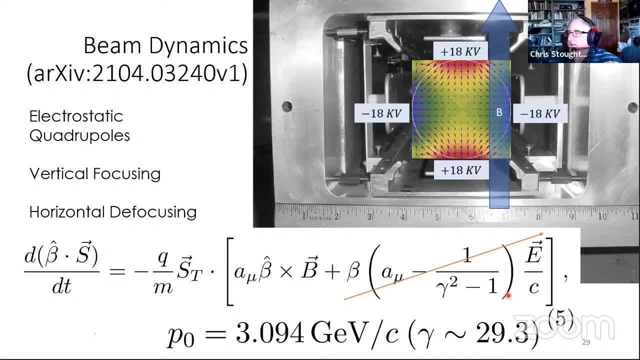 This is another fun homework problem to give to graduate students. Make an excellent homework problem to do, But anyway it turns out there's this so-called magic momentum where the nominal value of the anomalous magnetic moment is canceled out exactly when gamma is about 30.. 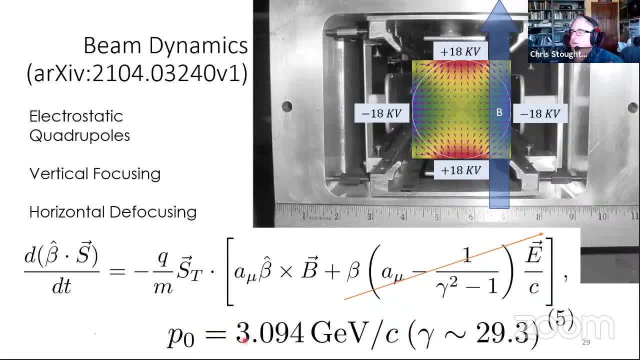 So if you have a momentum of about three dB, this correction is greatly canceled out. Then you just have to worry about the momentum that is above or below this by a fraction of a percent. So you get a lot more precision by going into the magic momentum. 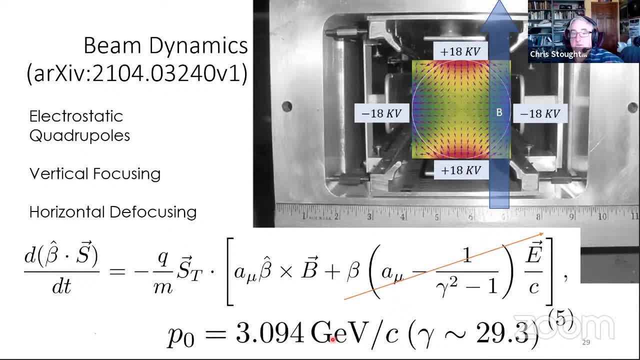 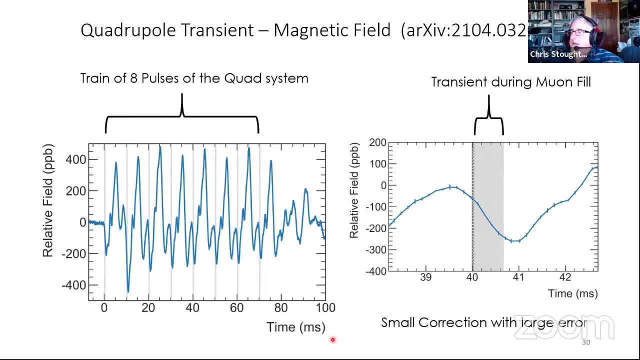 That was the huge enabler for the Brookhaven experiment to be able to do so well. Just another fact of life is that things move, And when metal moves in a magnetic field, it's a magnetic field. It induces its own currents, any current which? 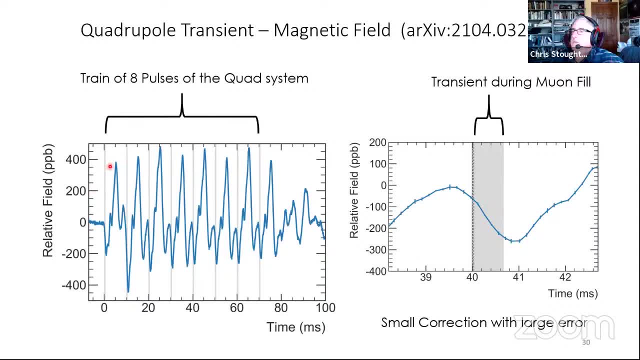 counteracts the magnetic field. So here's an example of the eight pulses that come from the accelerator all at once Each time you turn down the quad system. so you got less focusing, So the beam will blow up and hit collimators and stop. 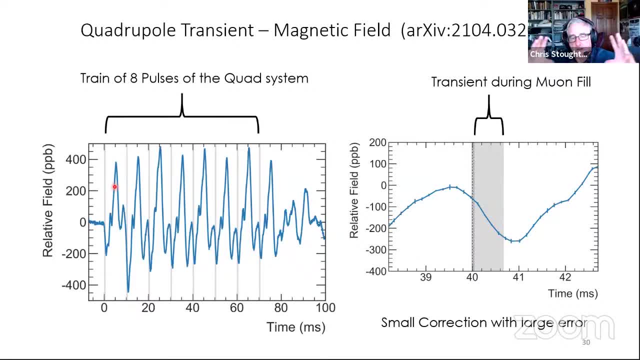 So you have a nice well-defined beam And then you turn up the quads, You squeeze that into your storage field And then you do the measure. Well, in the process of doing that, you've induced mechanical vibrations in the field. 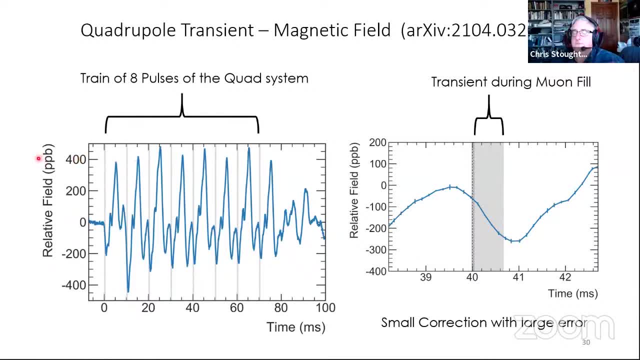 And they'll give you OK. it's only 400 parts per billion, So it doesn't change it by much. But in the precision game you've got to worry about that. Lucky for us, it always caught it going the same way. 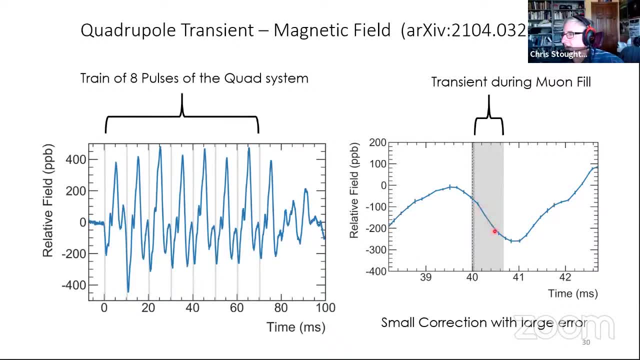 And this is as we sample the magnetic field during the fill. So, as a function of time, you put in a little correction And that's a small correction with a relatively large error, And this is one of the things we're really working on the measure this day. 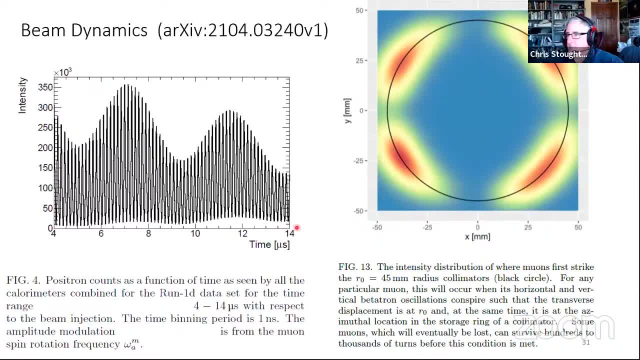 And then beam dynamics. The beam moves all over the place And you have the so-called coherent betatron oscillation With that hula-hoop effect. you throw in to kick it, it never really settles down. So you see, the positron counts are much more accurate. 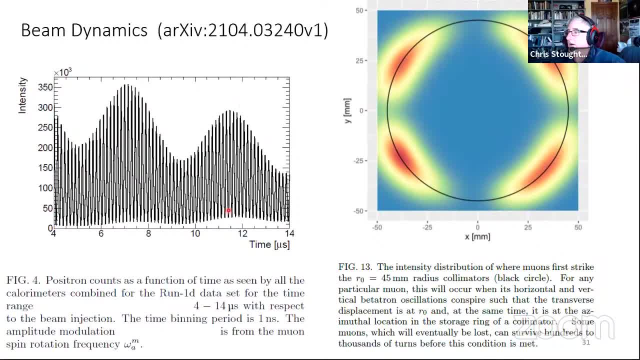 They're modulated also by these other coherent processes And it gets to be a real mess. You also have lost muons, So when they hit a collimator they're taken out of the sample. Turns out your probability: you'll hit a collimator. 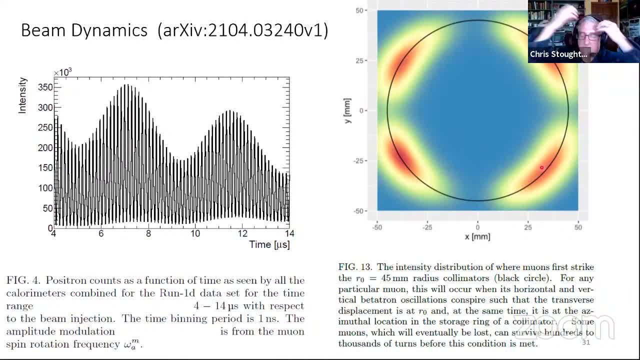 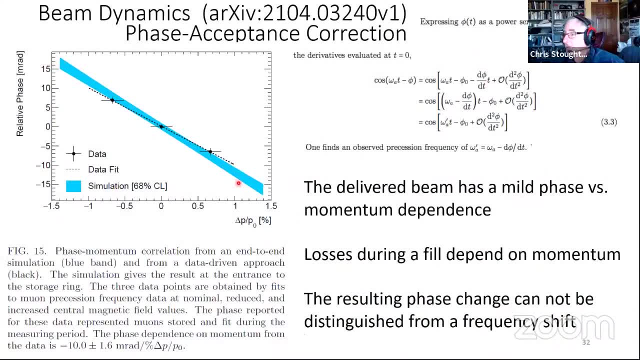 depends on your momentum, which depends on how much you precessed, So that's going to bias your effect. That's another reason to take that. And finally, the phase correction Right. So the phase of the muons coming in. 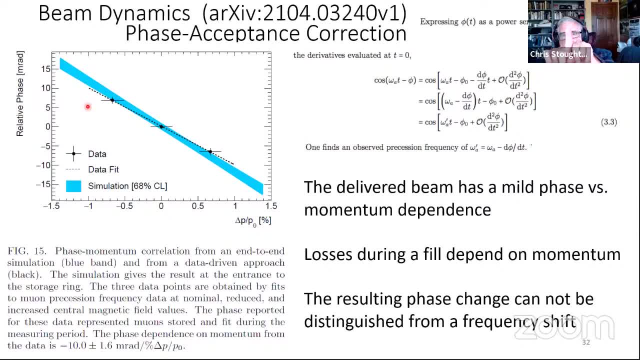 I told you they were all lined up exactly. But don't forget, the accelerator had the steer, the beam get it to us right. So when they steered it they used magnets And that caused a little bit of precession as a function of momentum. 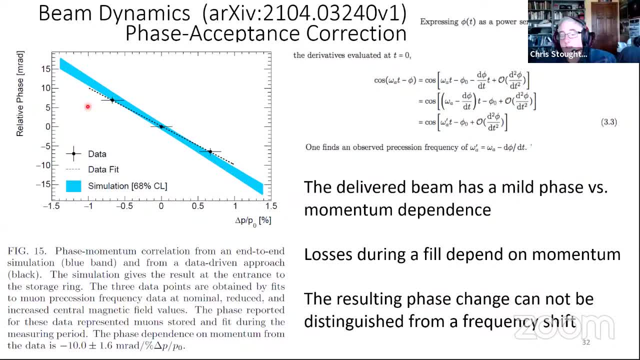 So your change in momentum is going to have a slight phase shift in what's going on And if you're, let's say, linearly losing as a function Your frequency, your number of lost muons, that change in phase effectively is a change. 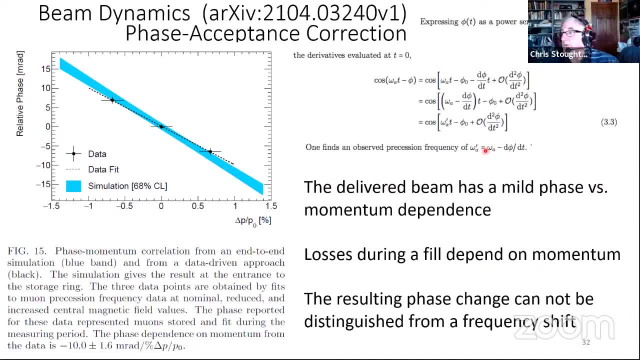 in your precession frequency, So you got to take that into account too. So all these things are little things you don't worry about when you begin, But when you're getting down to parts per million calculations, you got to do it right. 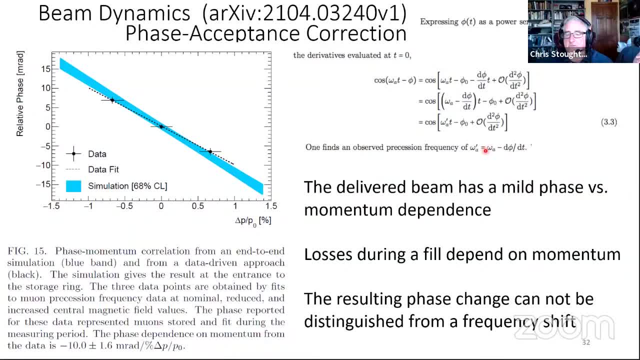 Each one of those analyses in the last four slides- or so I did. there are at least two PhD theses And years of work going behind each one of those, So that's why it takes so long to do this experiment. But anyway, let's hope. 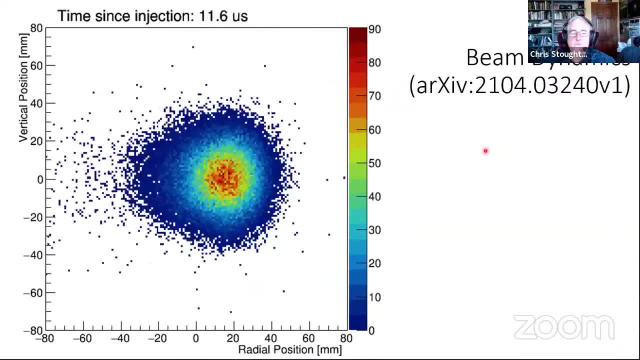 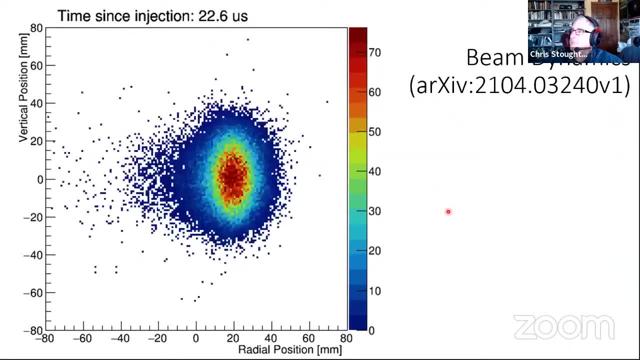 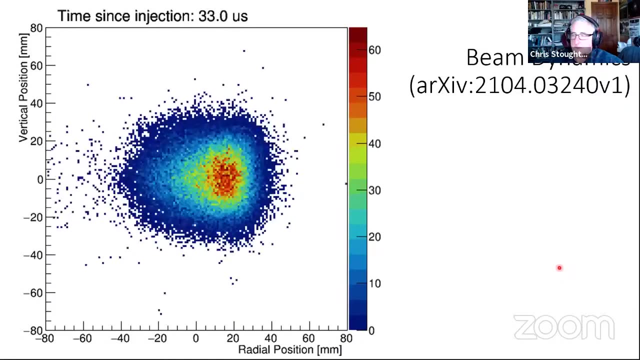 And just one more thing just to convince you that beam dynamics work. This is one of my favorite pictures. This is going through as a function of time, of the fill. This is measured of where we saw the decay tracks coming from. Decay vertices coming from, based on the track. 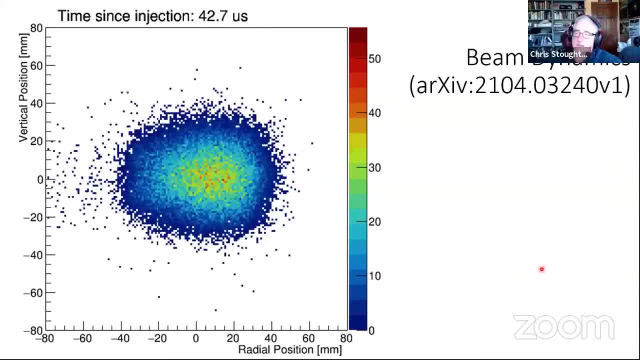 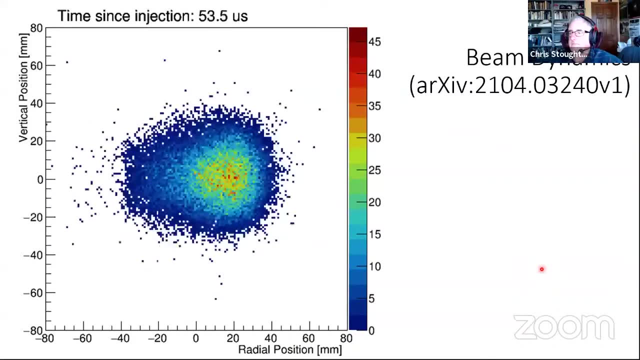 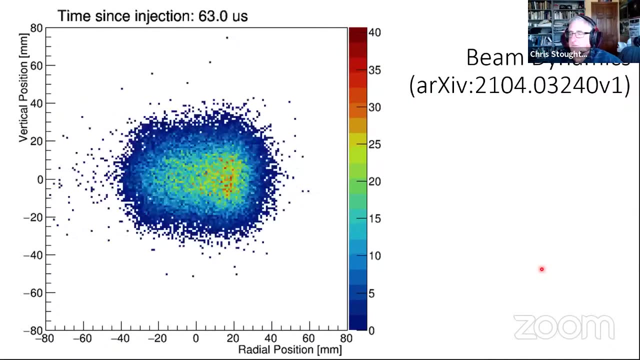 And you're going. it's breathing in and out And the magnetic field is not constant across that region. So this is the convolution of the beam position with the actual magnetic field that you've got to get rid of. So if you ignore all those features and just take 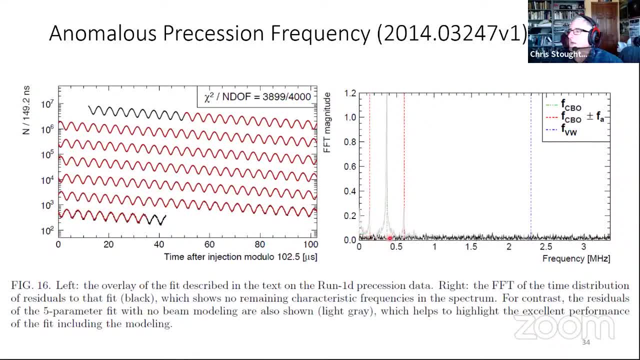 the Fourier transform to look at the frequency. you're completely dominated by these beam dynamic effects. So what you do is you do a 23 parameter fit which takes all these things into account. Some of them are modeled, Some of them are fit by loss. V1 data that we see. 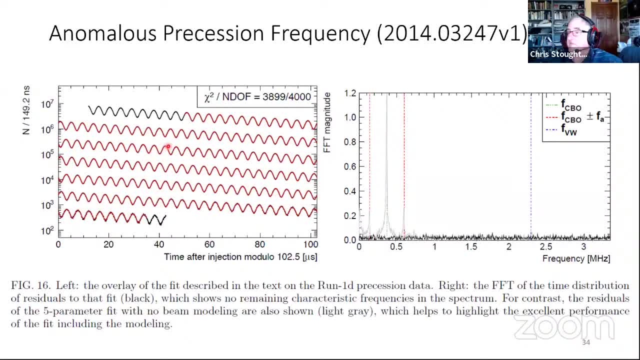 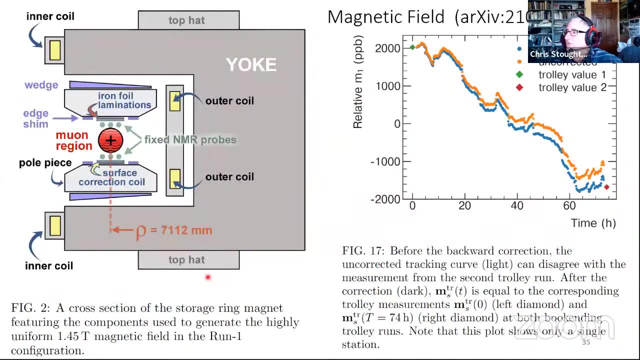 And one of the parameters coming out of that fit is the frequency you want, And the residual from that is this bottom one where the Fourier transform is dead flat. So it's taking all the effects into account. The magnetic field changes. That's a function of time. 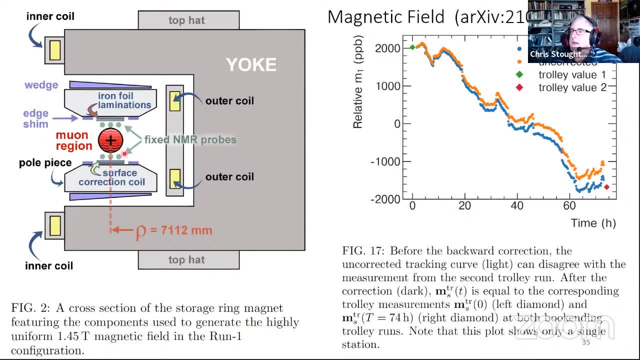 So every couple of days we stop and put in magnetic probes that go around the ring and measure it again. So you've got to take that into account. So all the data are corrected over time back to the nominal value of the magnetic field. 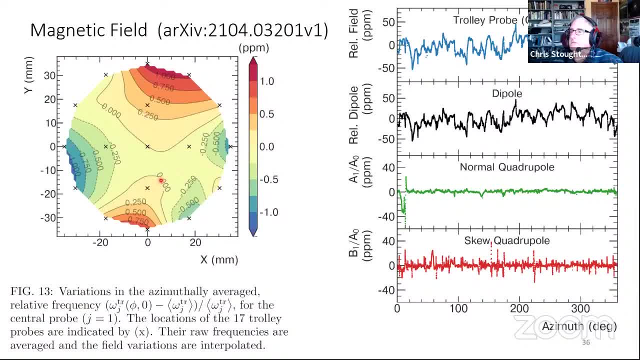 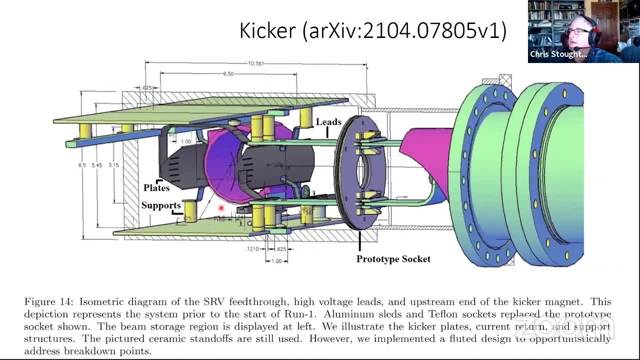 And the strength of the magnetic field inside depends. So this is the convolution. Here's the kicker that comes in and puts a current down and it comes back. And the reason it didn't get up to speed is because this is like 2 kiloamps at 55 kilovolts. 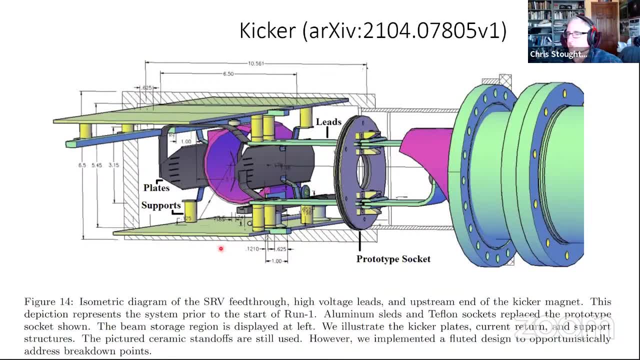 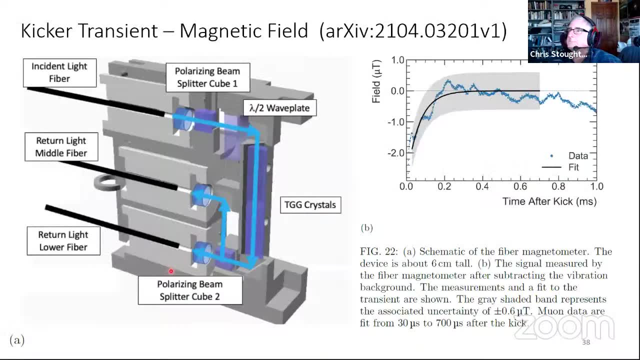 And things spark. I'll leave it at that- And we blow up the cables and didn't get the full strength. We kind of did some provisional rebuilding. It's doing much better now. And then measuring that transient field. you put a little QDD system in here. 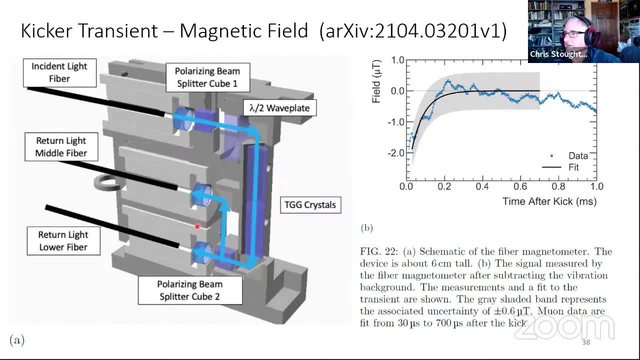 which would change the polarization of light depending on magnetic field. very clever way to measure this out And you can actually measure any current left behind by the kicker And that works out. And there is no significant magnetic distortion left due to the kicker plates themselves oscillating. 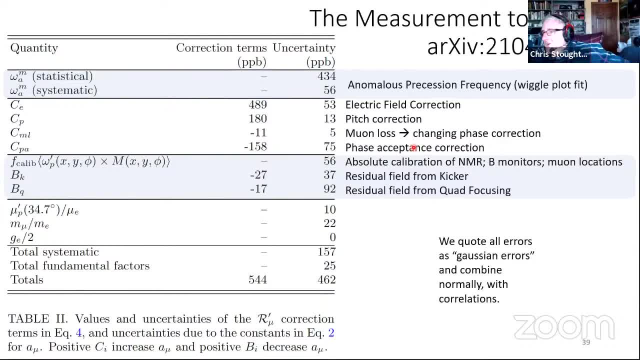 OK, so bottom line is you have this table of errors And this is now in our paper publishing the overall thing. This is sort of the shopping list And this gives you an idea of what the correction is to the value of r. 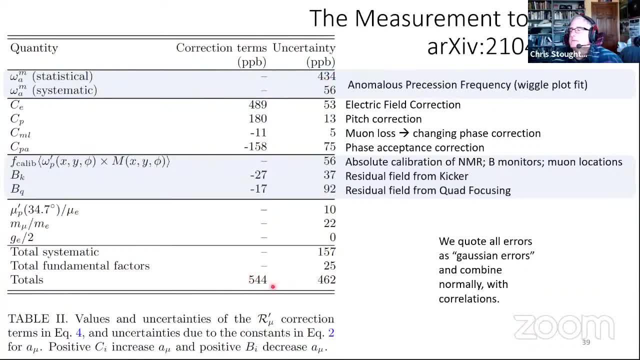 And this is sort of the uncertainty. So you're changing the central value by a little bit more than the sigma, And so the whole question is: what are the errors? And right now we're dominated by statistical errors which are pretty gaussian. 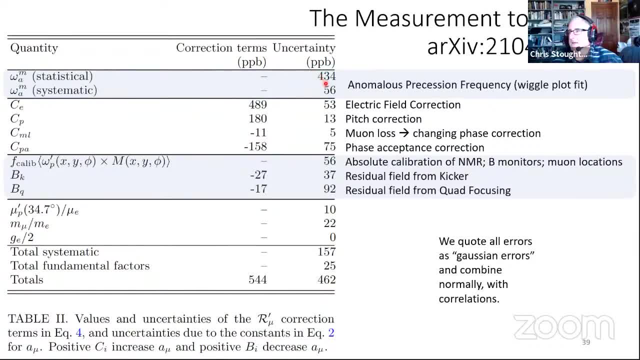 And if you look at these statistics, so I can sort of say, OK, these are all gaussian errors Or they're small enough that we don't need to worry about them much more. I hope to have a nice discussion about this later. 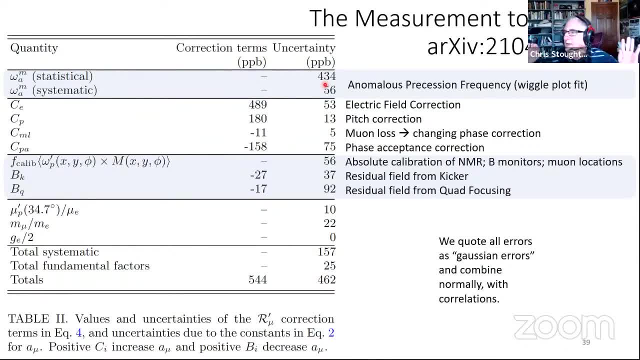 But what we said is: hey, we know how to combine gaussian errors And we're dominated by statistics now, So we're just going to do that because everyone can understand what we did. If you'd like to go back and do something more involved, 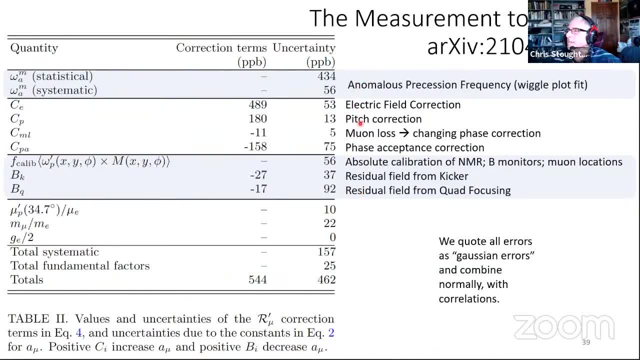 you're more than happy to do that, And this is the quick. It's a reminder of what each problem is, And the biggest ones are the electric field correction, residual from quad focusing, and then the absolute calibration and where the nuance are. 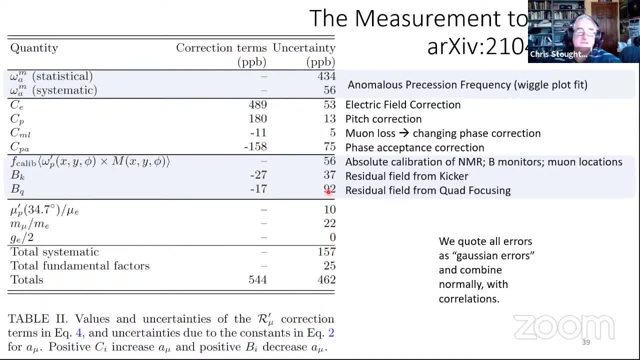 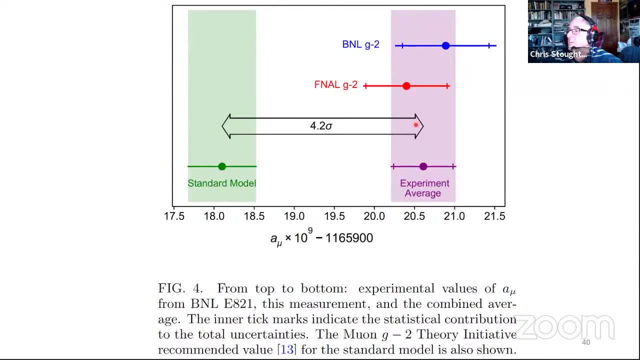 So next to other things, except for the strength, Yeah, so there's a lot of places to do work, And this is what's going on in run two and three. Anyway, you have to do all the math, do the combinations. 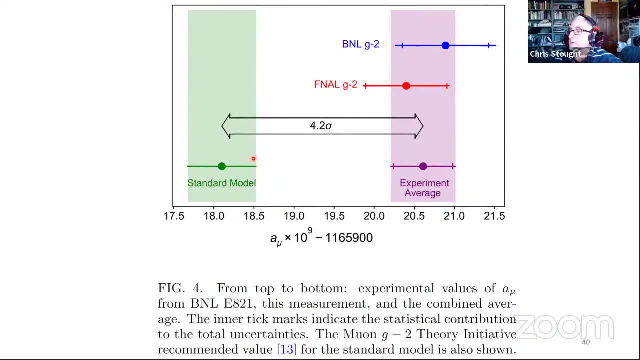 And this is a zoom in on the results. And here I've given you this is the anomalous magnetic movement times 10 to the 9th, minus this integer to give you the significant digits where it matters. So you can see, we're a couple of these units away. 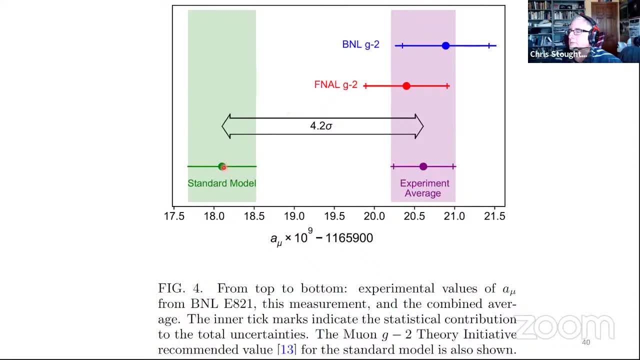 And that's 4.26.. This is the theory, This is us. It's amusing to see that, although our error bars got smaller than Brookhaven- because slightly better statistics- the mean value went down, which is OK. So what does it all mean? 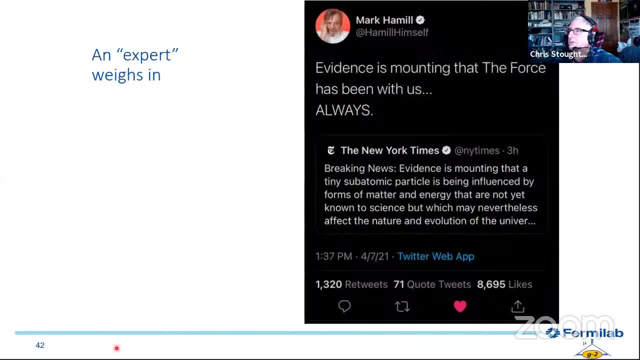 Raise your hand. if you don't know who Mark Hamill is, I think you may proceed. Thank you Good. So the big conclusions. What are we to make of all this? First of all, the g minus 2 experiment works in Fermi. 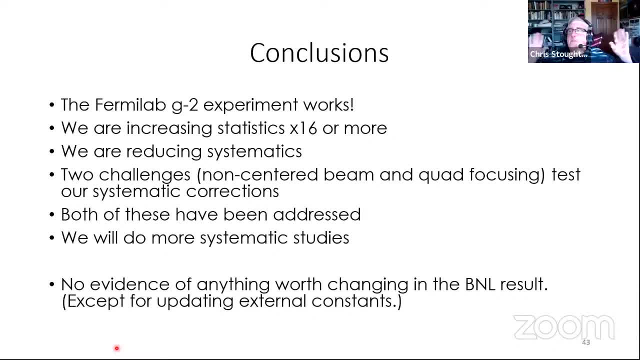 Right. All the systems work in Fermi Right. All the systems work in Fermi Right. All the systems work in Fermi Right. All the systems coming together, the darn thing works reliably. So that's the huge news. 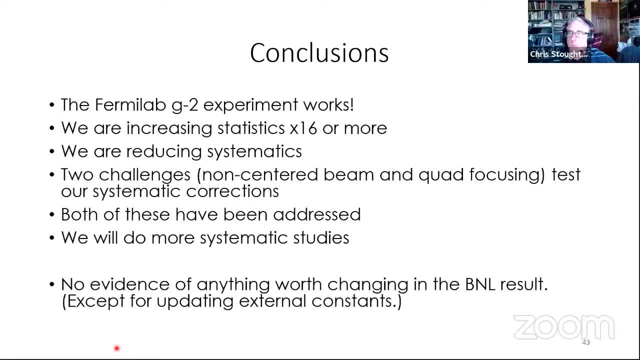 Give us more muons. That's exactly what's happening. We're going to increase the statistics by something like a factor of 16.. Of course, that depends on lots of things, But I chose to quote 16, because I can take the square root of 16.. 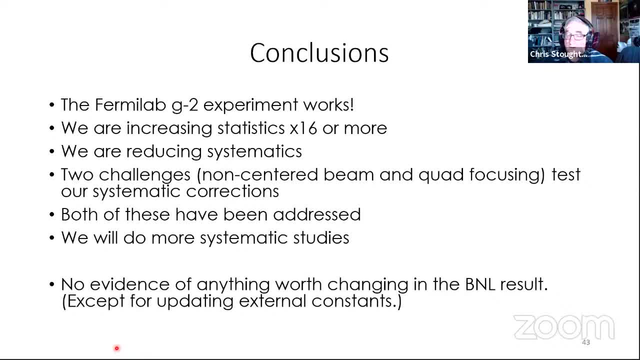 And that's 4.. So the error bar, the statistical error bar, should get something like four times smaller Right, And we're working on it, We're working on the systematics This first run, since we're underkicking. 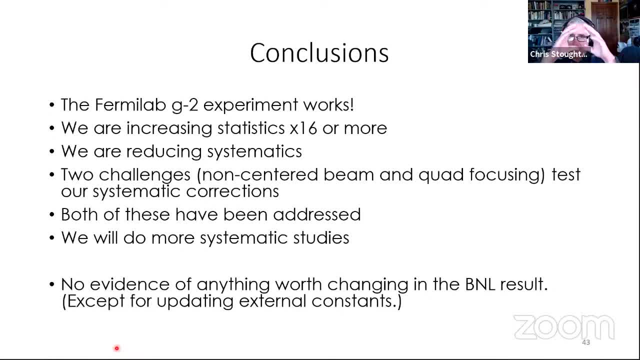 a lot of the systematic effects were worse. Now that we're centering the beam, where the magnetic field variation is more gentle, it's not going to be as bad, Right, In fact, the two challenges- non-centered beam and the quad focusing beam- not quite as good as it could be. 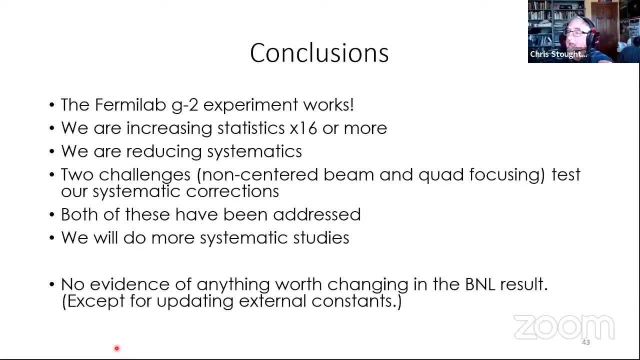 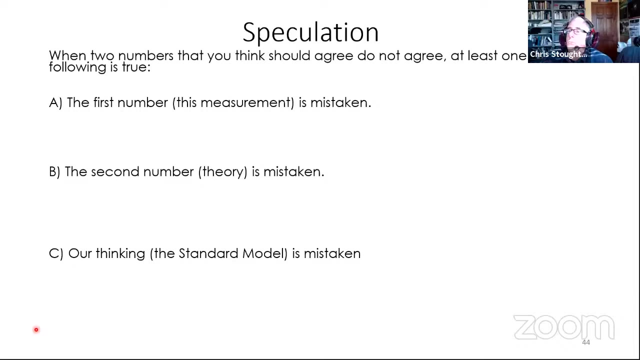 really tested them Right. And probably the biggest sigh of relief I heard was from the people who on both experiments that we saw nothing, that they did wrong, Right, Anything worth. there's nothing worth changing in the work. OK, So now we enter the realm of pure speculation. 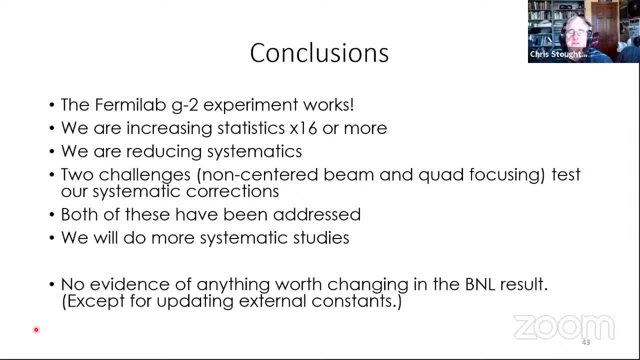 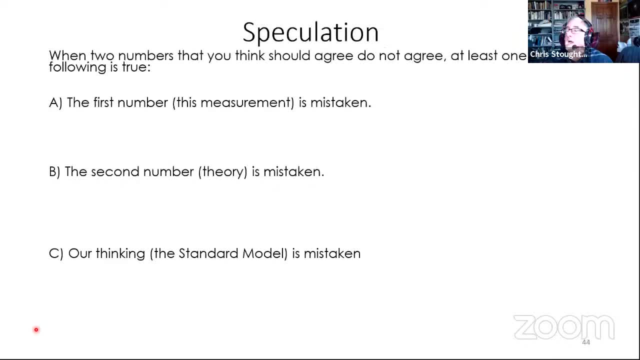 When two numbers that, so in a certain sense I should formally stop the talk. This is all solid ground, But what fun is that? Let's Right Right. If two numbers don't match either, the first number is wrong. the second number is wrong. 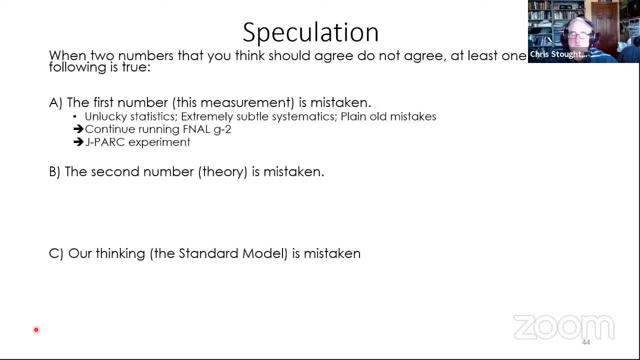 or your thinking is wrong, Right. So to fix the first number being wrong, it could be we have unlucky statistics, Right, Or some extremely subtle systematics, or just little mistakes, Right? So we're going to keep running g minus 2.. 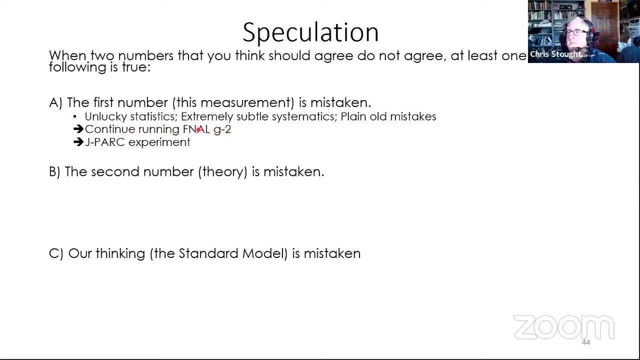 It's a collaboration of young, smart people that are working hard to find mistakes. good for them. And Jay Park is running a completely independent experiment. I'll show you a picture of that later. You've got to repeat the experiment right. More fun for me to think about because it's. 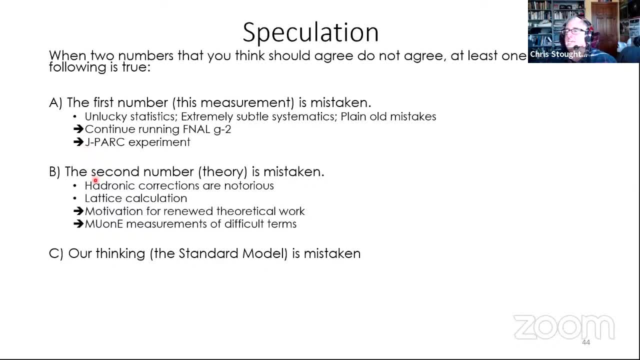 someone else's problem is that there's a problem with the theory, right, I mean hydronic calculations are notorious to me. There are lattice QCD calculations coming out which are giving what they claim to be are different values than the other theory, which 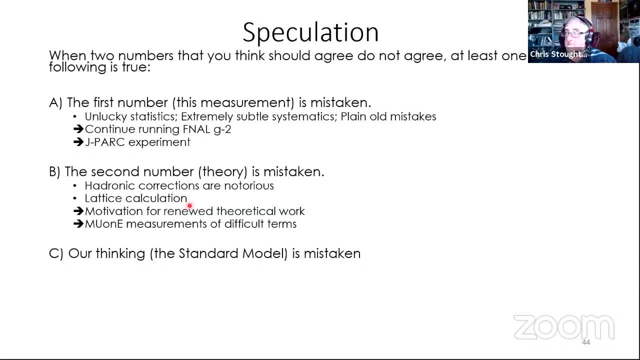 is more in agreement with experiment. That's extremely accurate right now. But you know, the good news Is there's motivation for more theoretical work, And some of the terms in the theoretical calculations are what they call database calculations, which means, rather than calculating, we're. 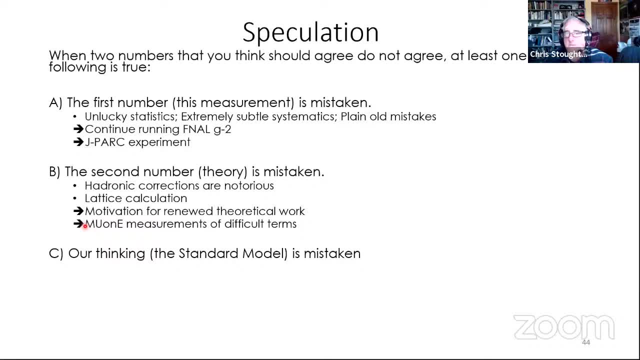 taking some of the form factors from scattering experiments, So redoing those experiments. in fact, there's a CERN collaboration that's prototyping now, mu on E, that's going to go do those measurements better. Now, of course, the fun thing to think about. 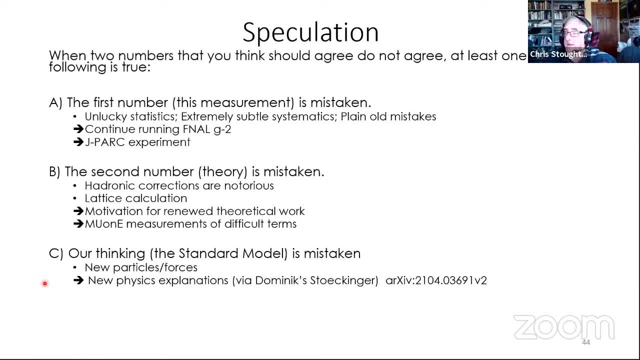 is that? oh, we found something wrong with the standard model. Yippee right, There's a new particle, There's a new force. I still think the most sober description of the state of play is Dominic's paper. he wrote now, back in April, I think. 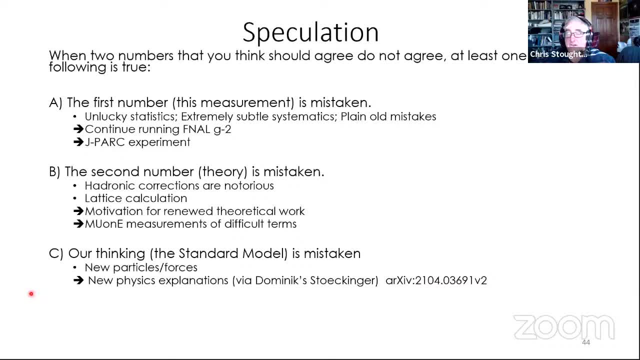 where he points out that hey, there's still plenty of room for supersymmetry. Go ahead and speculate what you want, But kind of normal beyond standard model physics, there's still plenty of room for that. But if you want to go crazy and talk about luck, 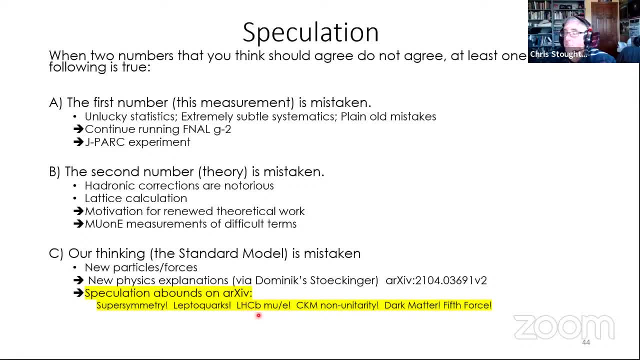 though quarks, or say that there's combination. there's some correlation with LHCb. their muon electron anomaly is a few sigma right. The CKM matrix is not quite unitary, and it should be. You've got dark matter. 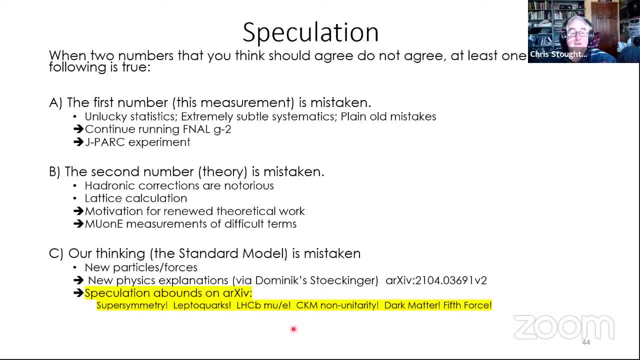 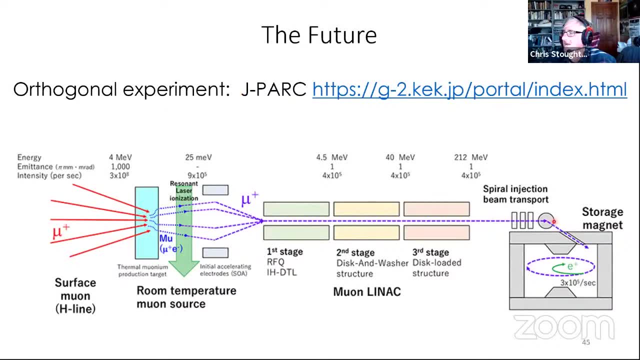 You've got the fifth. fourth, Put your favorite speculation in there. Read the archives and have fun. OK, here's the J-PARC experiment. They do basically the same thing, except their storage area is one big empty evacuated surface. 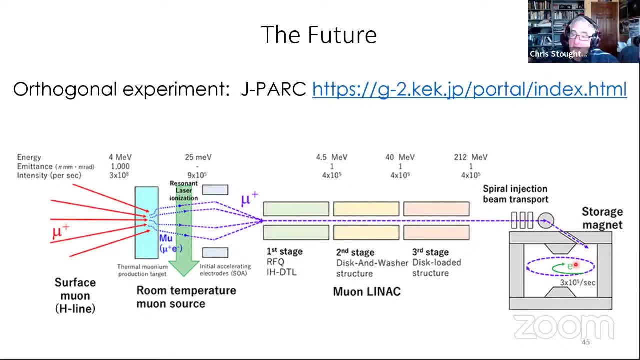 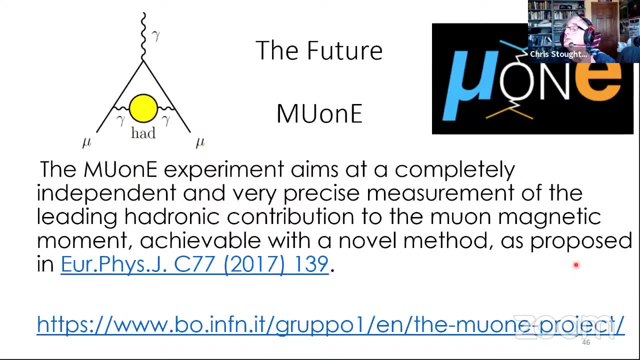 OK Area volume where they allow the muons to precess and they've got a 3D view of all the. That's a lot less systematics, but the problem is getting the flux high enough And the muon e-experiment is here. 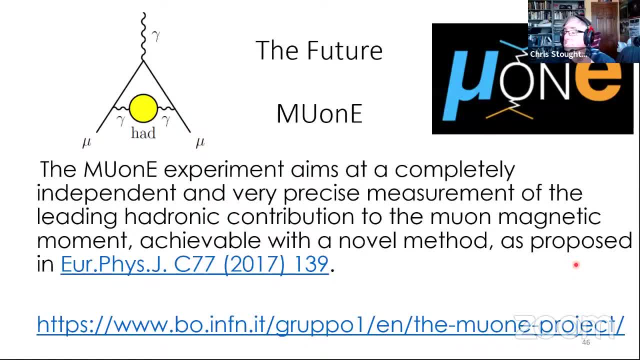 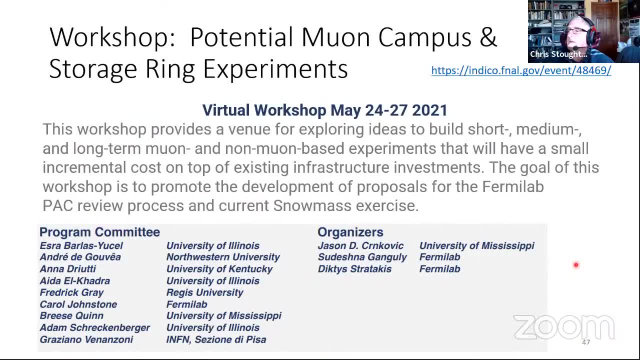 They've got. if you want to join a new experiment, join it. Plus, it's working with Italians, So you get that good. There's all sorts of talk. It's permanent. What to do with the ring? Should we run a new plus?